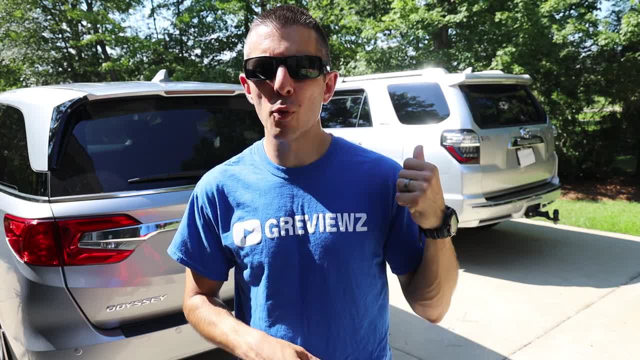 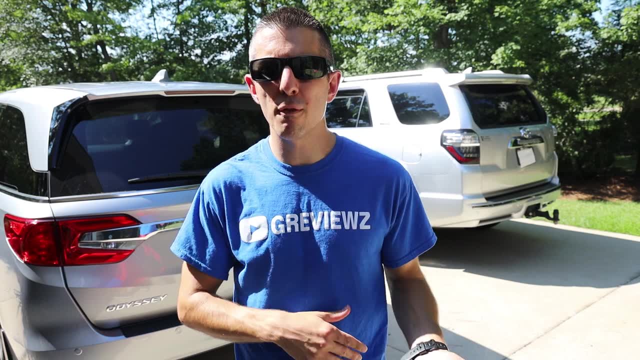 also because they're in the same price point. All right, if you go for a 2020 4Runner Limited or if you go for a 2020 Honda Odyssey, they're both going to max out somewhere in the neighborhood of about. 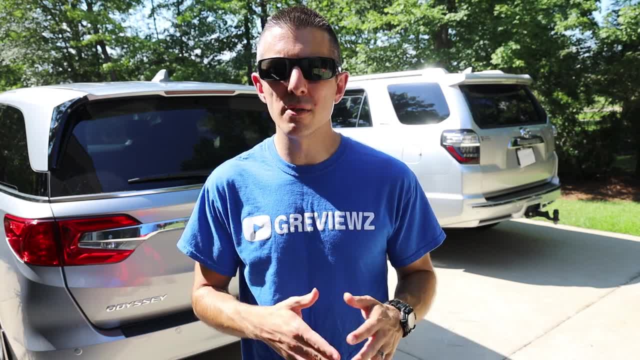 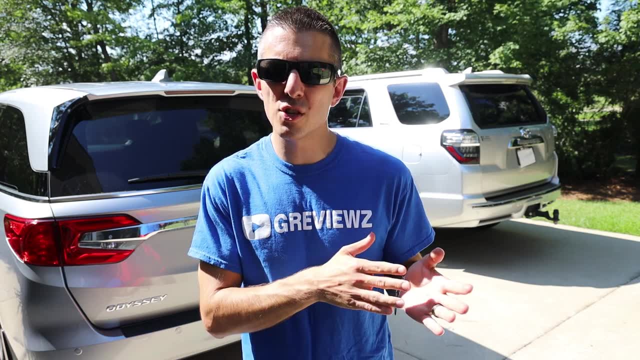 $48,000, maybe $50,000.. It all depends on where you live, But both of them represent about the same price points and what a lot of people are looking for: A mid-sized to large SUV and a minivan. That's what the majority of what families are looking for. Obviously, people get passenger cars or trucks. 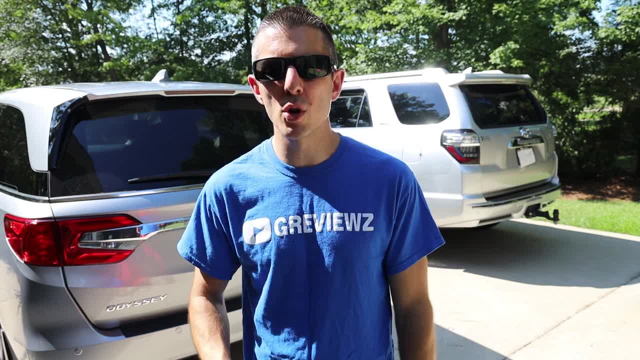 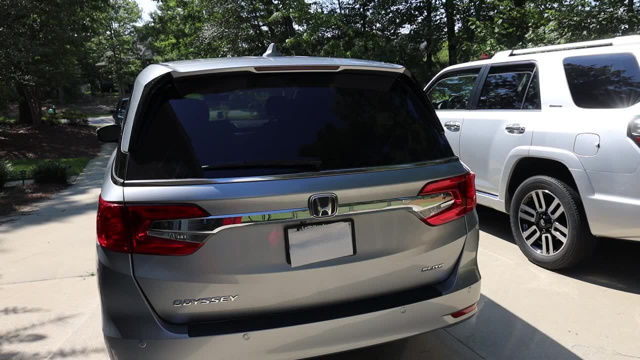 But the good majority of families like these two types of vehicles. So we're gonna start with the rear storage. We're gonna start on the minivan first and then we'll go to the 4Runner. There are a total of three ways to open this back door on this Honda Odyssey. 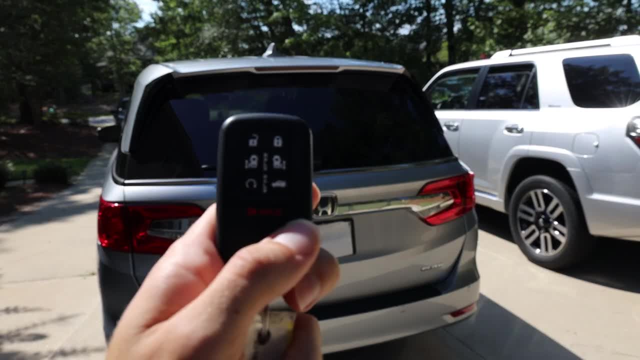 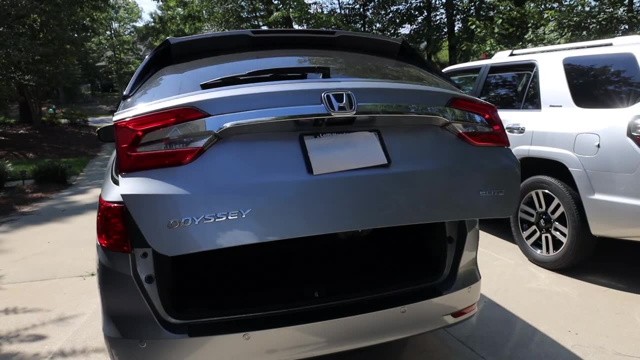 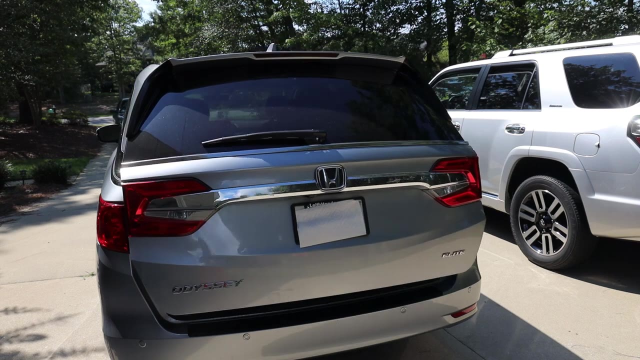 The first way is going to be the key fob method. All right, this button right down here. You just push it, It opens the back. We're gonna shut it. There we go. Second way is going to be with your hands. 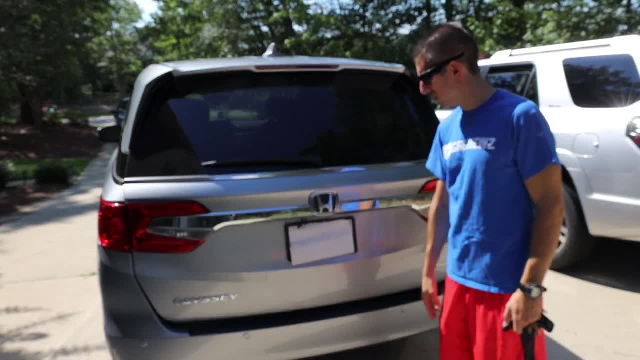 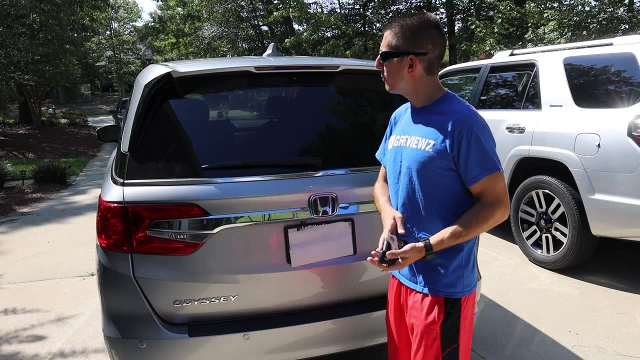 There is a pressure activated switch Switch right down here. Obviously, open it up like that. There we go, And then the third way is going to be foot activated. I always have a little trouble with this. My wife seems to do it, no problem. 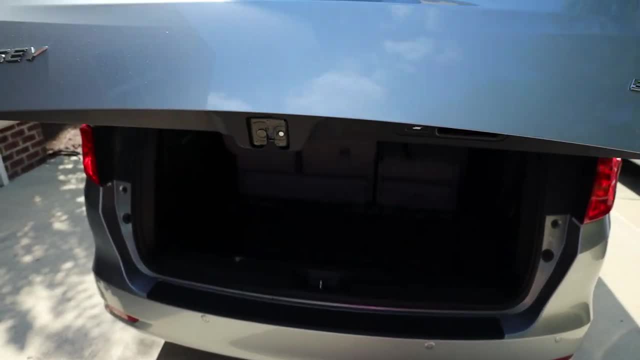 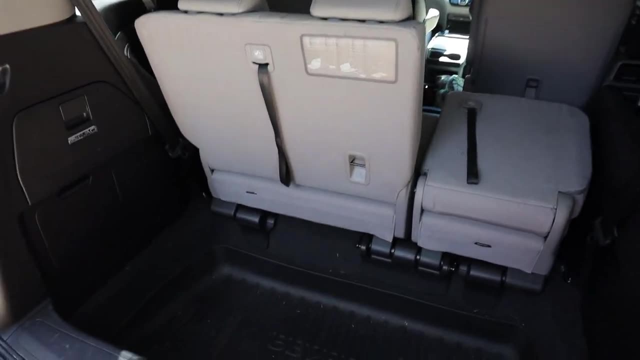 There we go. Just a certain spot you got to be at. Alright, those are three ways to get in the back. Once you're in the back of the Odyssey, you actually have a good amount of storage. It is actually quite a bit more storage in that 4Runner. 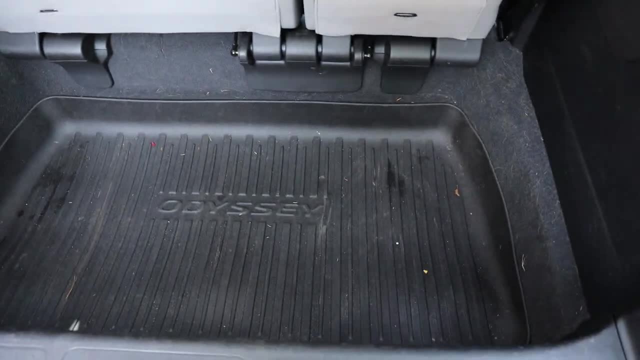 I do have a tape measure. I'm going to do a couple of measurements, but first I'm going to show you all the different configurations back here. All right, so we're going to pull this up. This is the third row seat, okay. 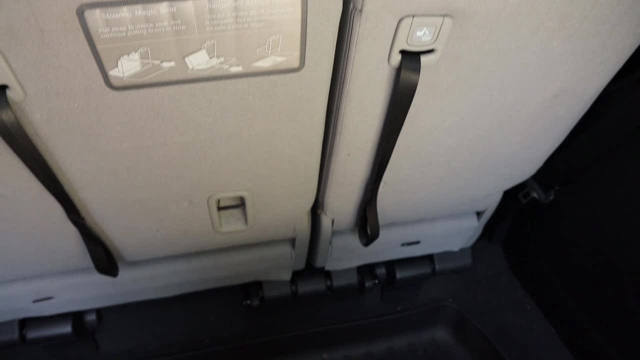 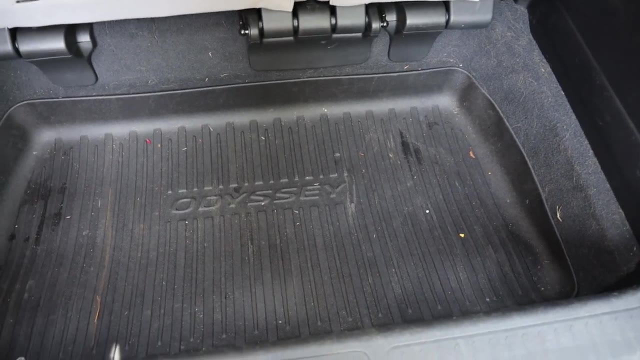 It has obviously placed three seat belts, It's got three headrests and you've got this really nice deep storage. This is where pretty much my wife will put all of our groceries if she goes grocery shopping. or you can put either strollers or whatever have you in the back. 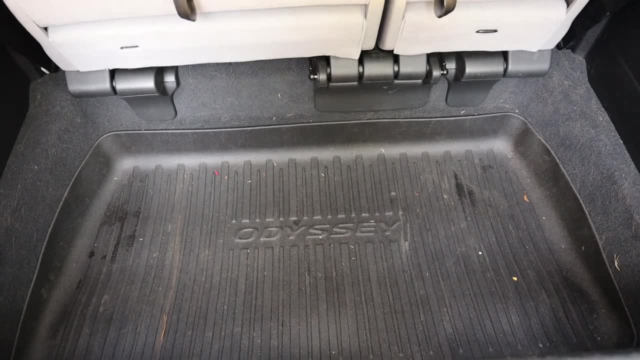 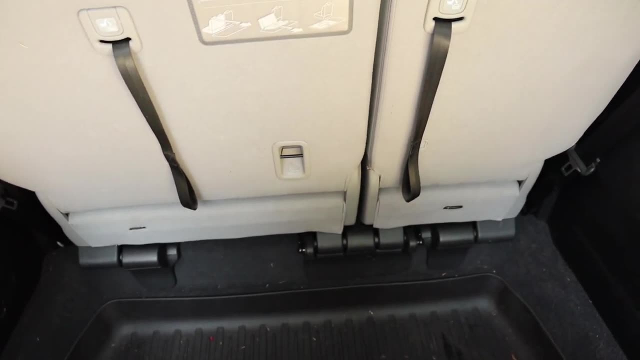 I got a couple items I'm going to throw in here in a second just to show you kind of a comparison between this and the 4Runner. Alright, this particular van does not have any sort of power, rear seats or anything. It's all manual. okay, All you're going to be doing is pulling on these. 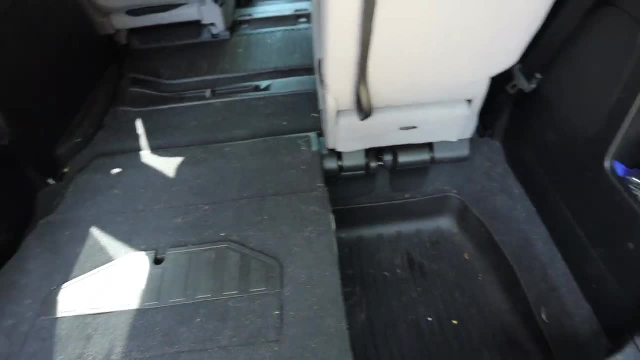 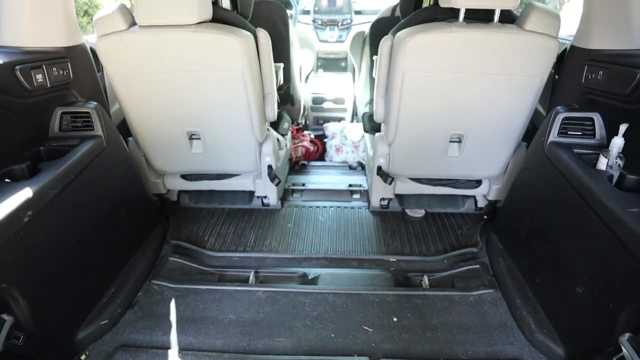 Alright, see that, fold right down in there. Alright, super easy. Alright, see that. It took me no effort whatsoever. As you can see, there is a ton of storage once them seats are folded down. Okay, a ton of storage. 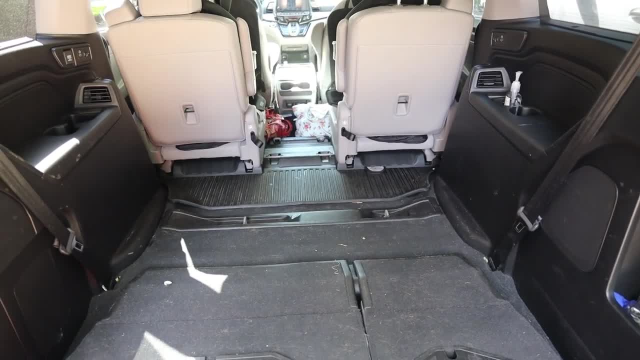 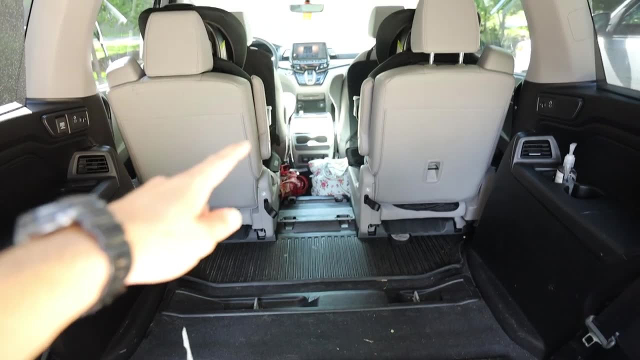 Apart from all the mess in here, I didn't tell my wife I was going to video her van, but this is just kind of how it is, Alright. so we are a family of four, so this configuration right here on a trip is perfect. 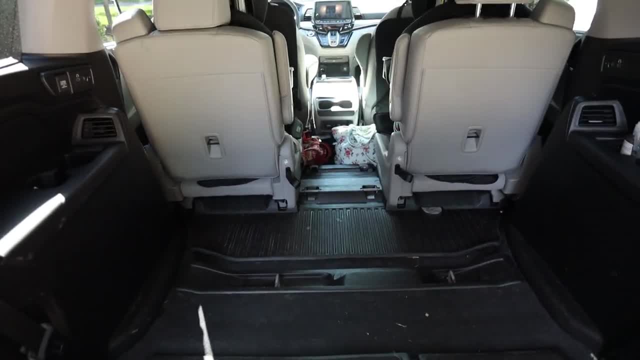 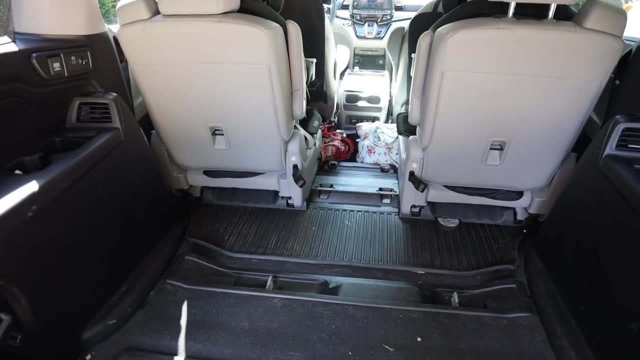 We've got the. it's four captain's chairs. alright, There is a center seat that goes right there. You can see the bars are clips in, but we do not use it. I'll show you in a little bit why. Alright, I'm going to throw a couple items in here, just to show you a size comparison. 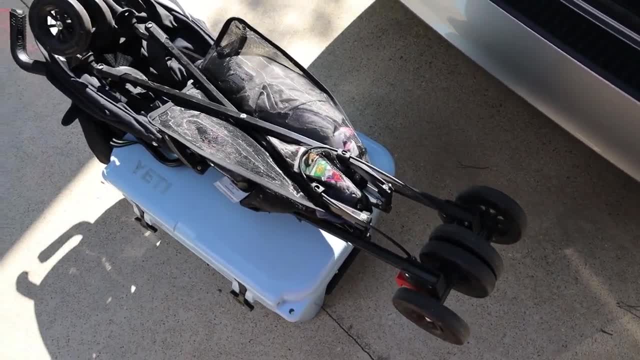 The two normal items you would see in the back of my wife's minivan. So here we go. This is it, Kind of a large umbrella stroller. Obviously, if you are a parent, you know what an umbrella stroller is. 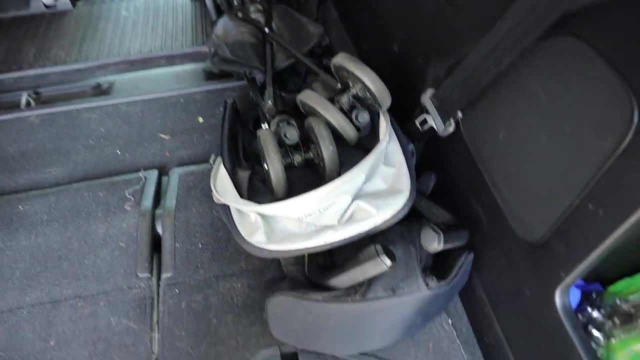 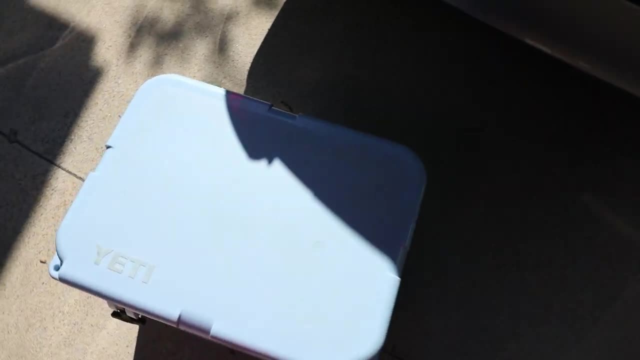 So if you want to throw that down all the way to the front, it shows you kind of how much room. This is about a foot right here. I know it's hard to judge. Alright, the next item. Yeah, this is a Yeti Tundra 35, so not the biggest cooler, but it's definitely not the smallest cooler either. 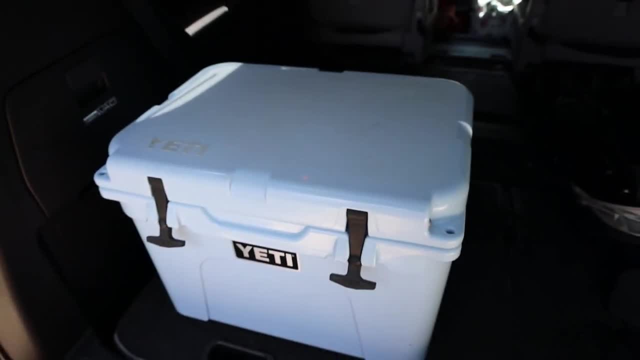 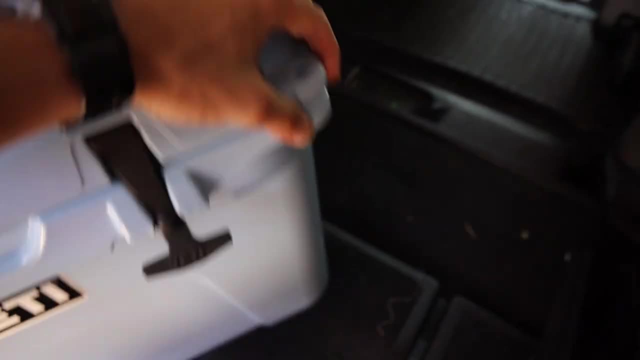 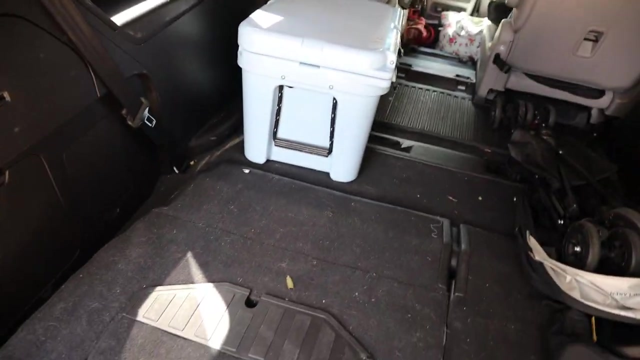 So we're going to put that in here like so, Alright, so there's that. Obviously it's got a lot of room And if you turn it around, the lengthways, Alright, there we go, Alright, so that's about. from here to there is about three feet. 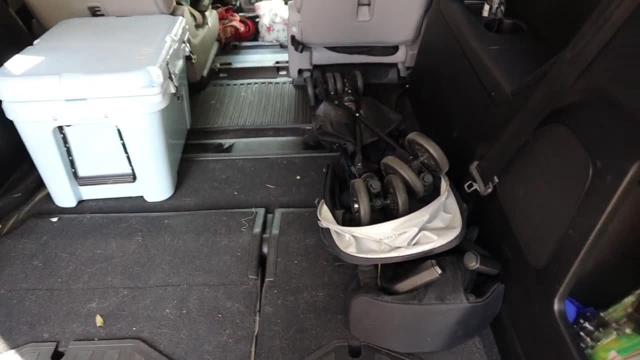 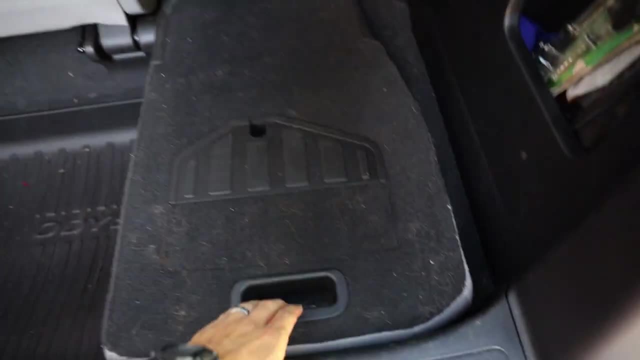 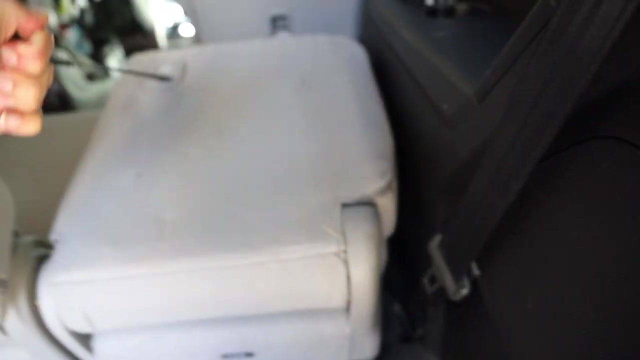 So that just kind of shows you how deep this van actually is. Back up again, It's all manual. As long as you can reach these, you'll be just fine. Well, I kind of went too far there. Alright, that's the normal position of the rear seats. Obviously, like I said, there's a great storage down below. 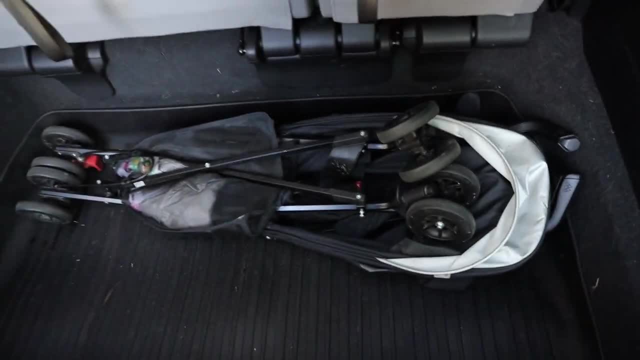 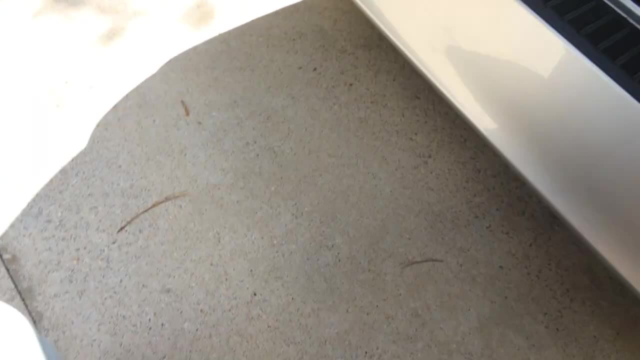 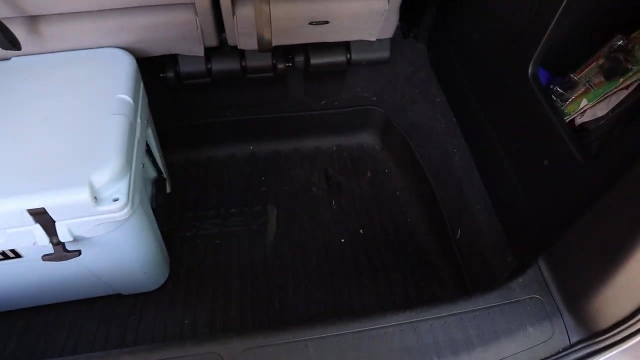 Here's what it looks like with the umbrella stroller. So you still got a lot of room in there and then take that out And I'm going to throw the Yeti in there. Alright, there you go Again. the van has great storage On to the 4Runner. 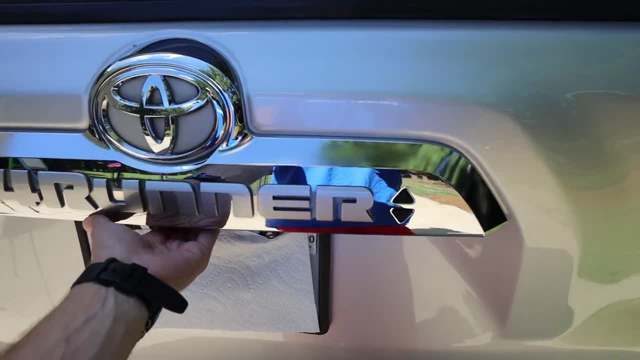 The only way you can get this Tundra 35 is to put it in the back of the van. Alright, so what we're going to do next is the tailgate. The tailgate to open is the lever on the back. Alright, here is the rear of the 4Runner. 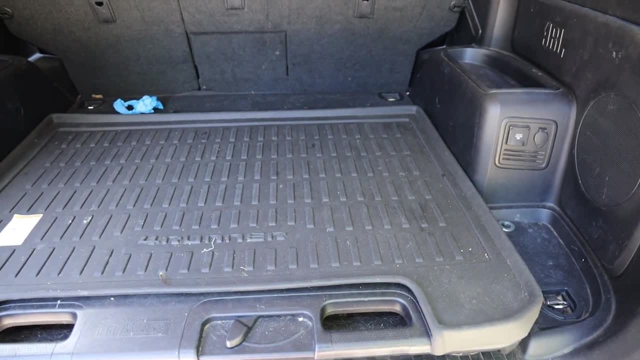 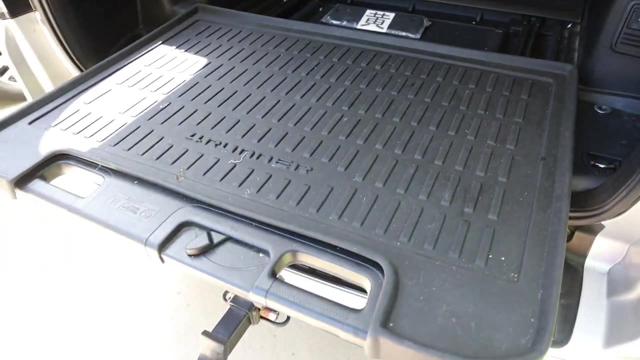 When we first bought this, we opted to just get no rear seat. We wanted the slider. Okay, this thing right here is a great feature. We use it as a tailgate for going somewhere. we like to sit on here like if the beach or someplace. It's great. 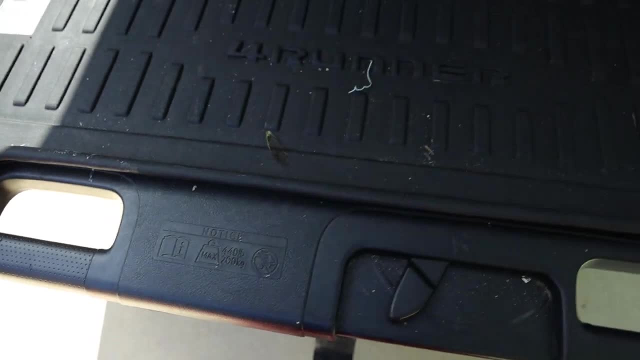 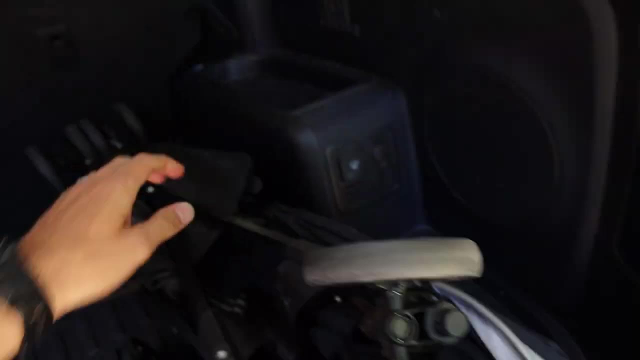 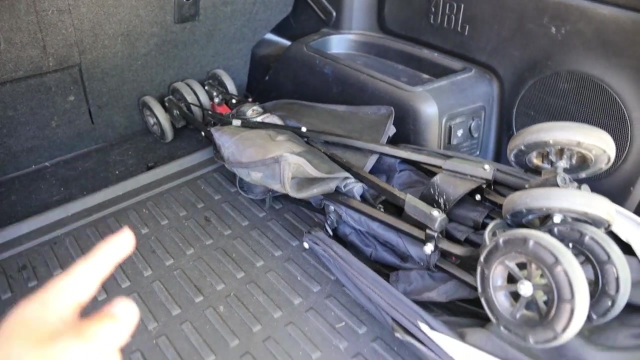 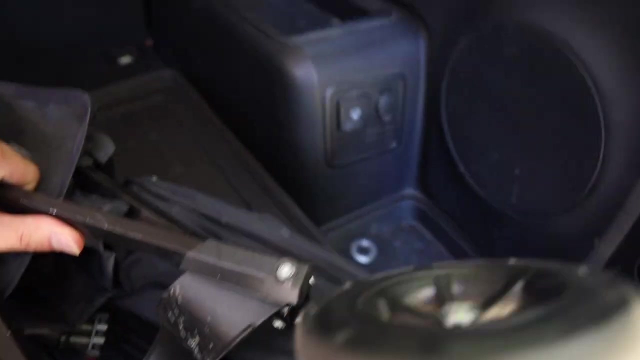 It can hold 440 pounds. You got the same stroller and cooler. We're gonna throw this in the back of the forerunner, Alright? as you can see there, that stroller is all the way to the back of the seat here And it's not gonna be able to close, so obviously with this particular item. This would have to be a sideways item. 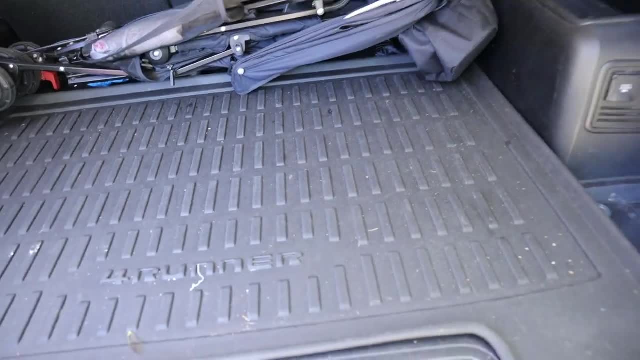 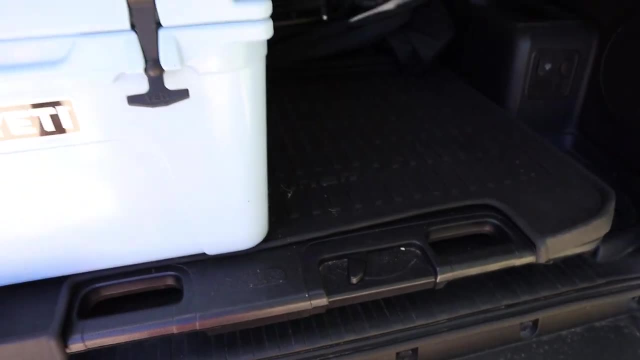 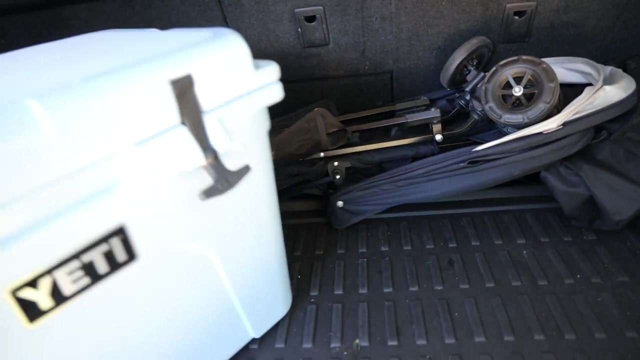 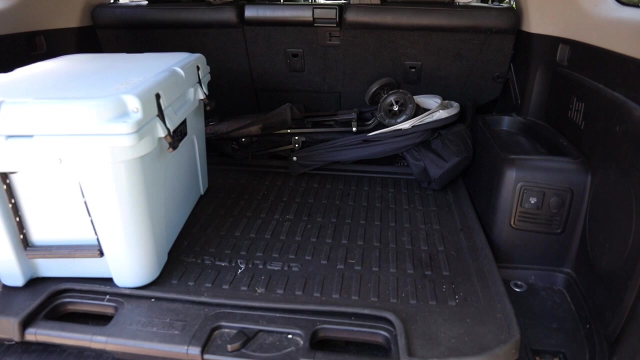 Alright, so def is gonna fit in there like that. okay, now Let's throw in the Yeti, Alright. Alright, that fits just fine. Okay, turn around sideways. All right, there we go, if it's just fine. So obviously you can definitely tell right off the bat: There's a lot more room in the van. 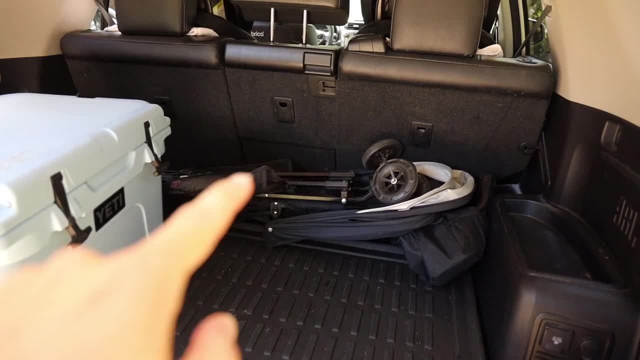 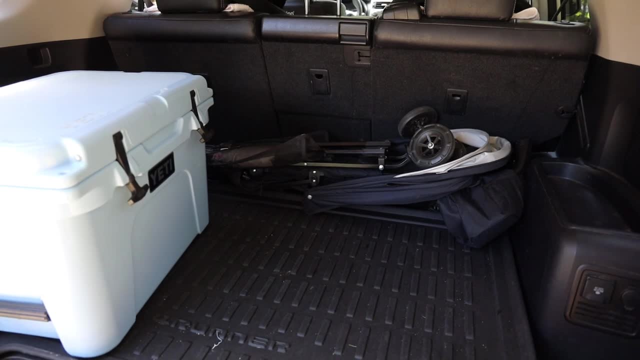 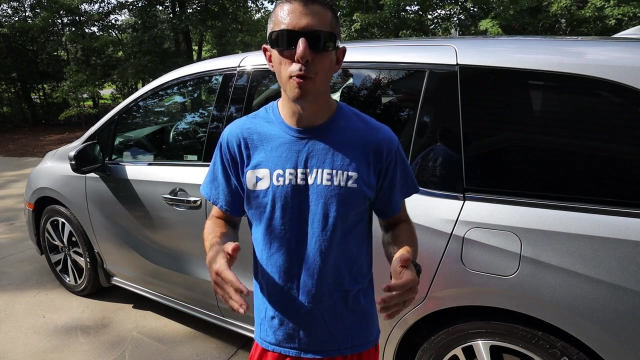 Obviously, if all you have is two or three kids in both The vans gonna Have a ton more storage. Okay. now, however, there is a benefit to the forerunner over the van. the most important thing on a family vehicle is obviously the Room for the kids. the whole reason why you're buying a family vehicle is because you're a family. 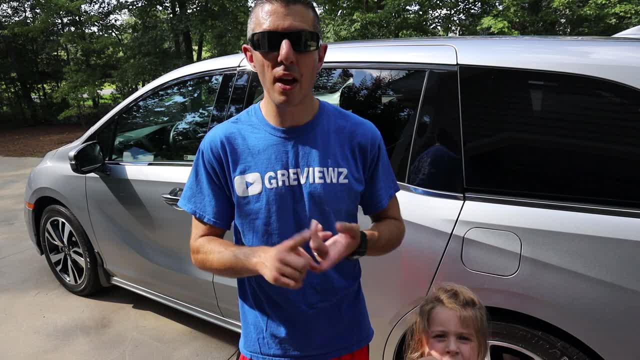 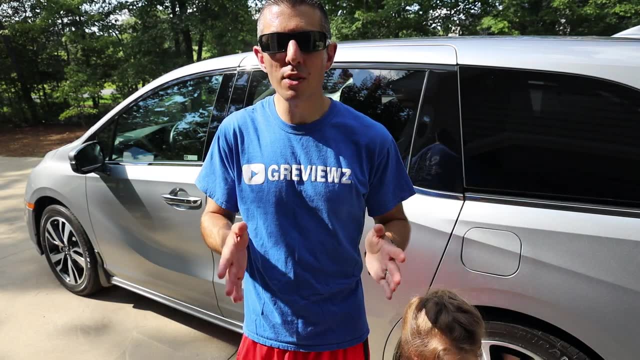 there's no reason why anybody would really buy this minivan unless they either had a Family, or if it was an elderly couple, or maybe someone is looking for something that has some storage, But the main reason would be to have some kids. so I'm gonna do a demo with my kids to show you the inside storage. 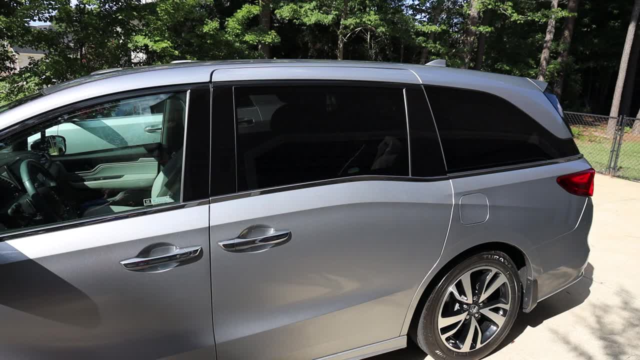 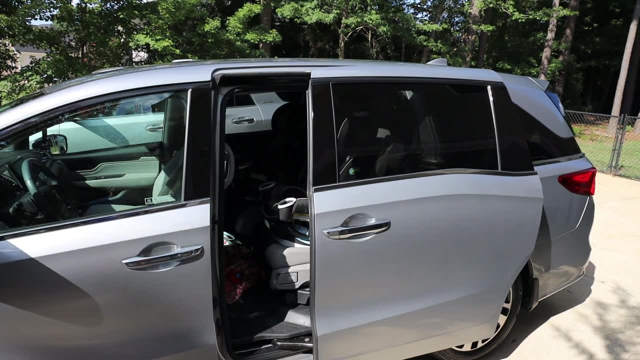 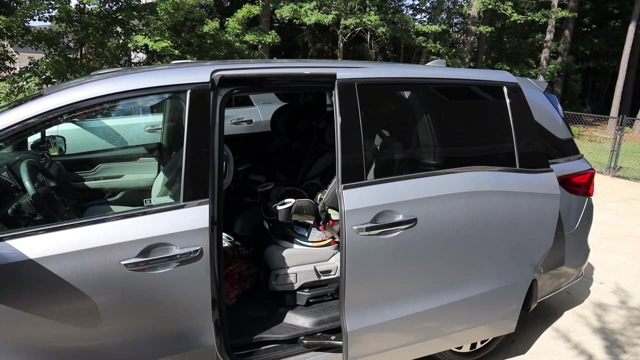 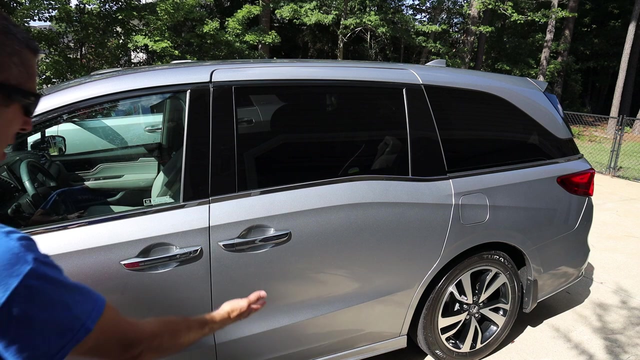 Where they're gonna be at. to get into the center section on this, that you're gonna have, Obviously, the key fob controls. All right, there you go on. that you can close it from the key fob, All right, then you have obviously the handle which does the same thing: opens and closes it. 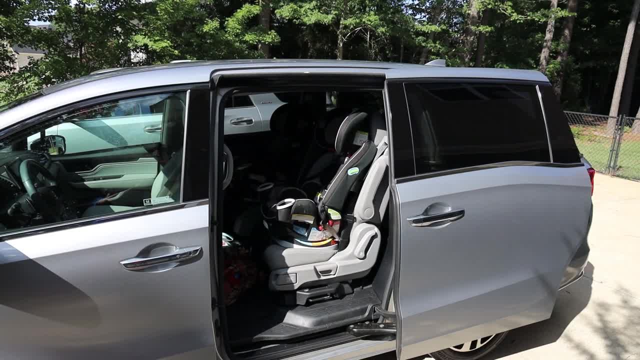 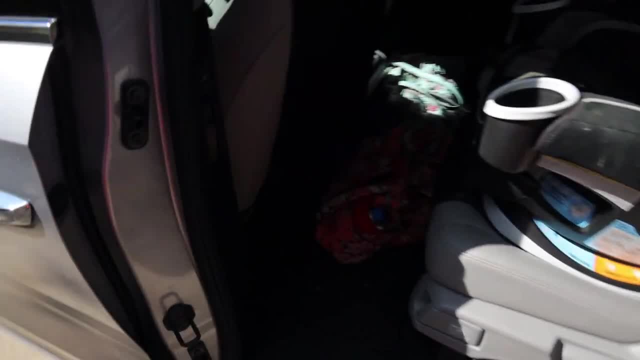 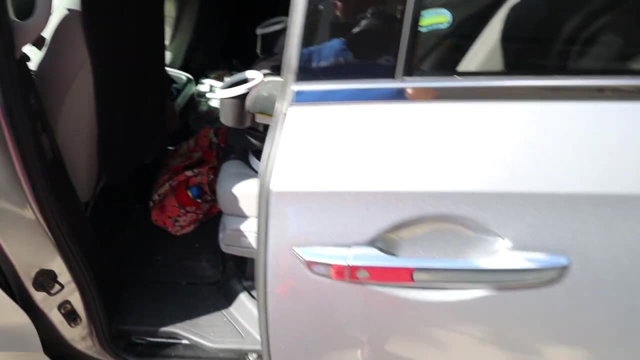 All right, I'm not gonna go by the closing it again. All right, got it off the tripod there. and then the third way is going to be right here. Don't know if you can see that or not: open and close, So you close, and obviously there's your three ways of getting into these side doors as well. 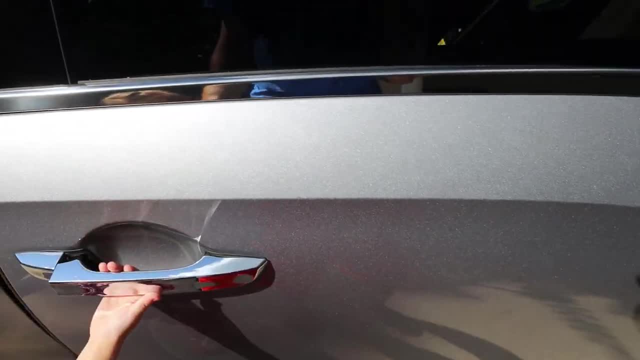 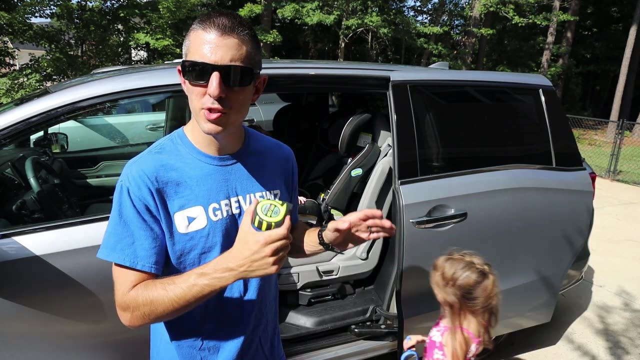 All right, Here's my girls here. We're gonna do a quick demo of some of the benefits to the minivan. in this shot, Obviously, you can see my girls running around here. I got a tape measure to show you the differences in the in the size of the sides and the headroom and such. 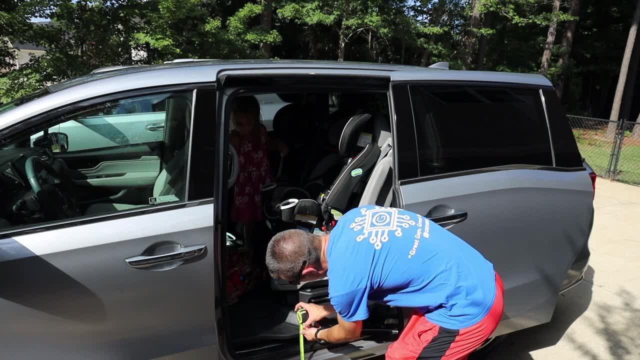 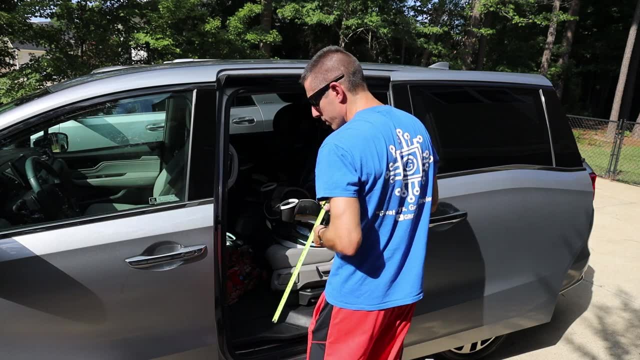 All right From the ground to the absolute first step that you can get into. on the side here is going to be 15 inches, Okay, so going from the grounds to this first step right here, I don't if you can see that on the camera. 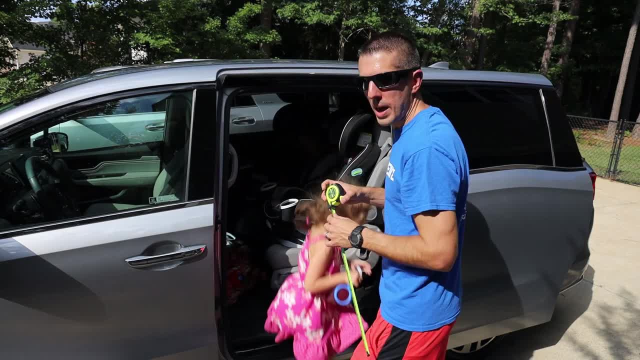 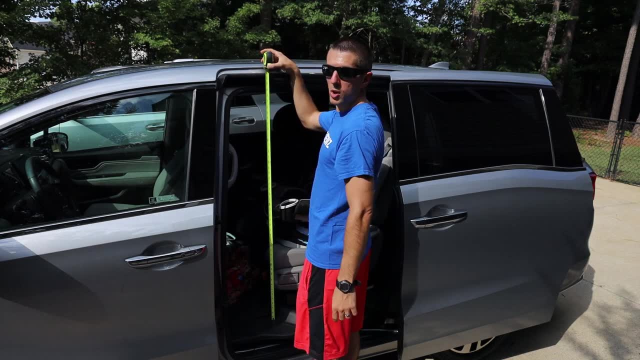 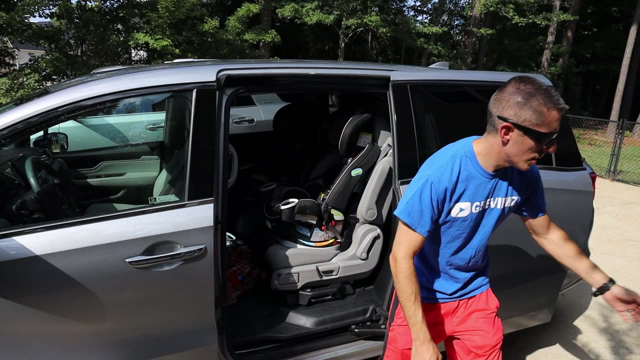 It's gonna be 15 inches. Okay, now the actual opening from the ground to the actual opening top is 45 inches. Okay, All right, girl, come over here, Come on, All right. so, for example, she's my daughter here, is four years old. okay, hop up in there. 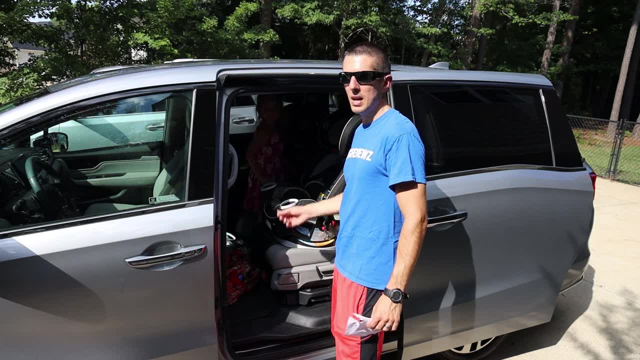 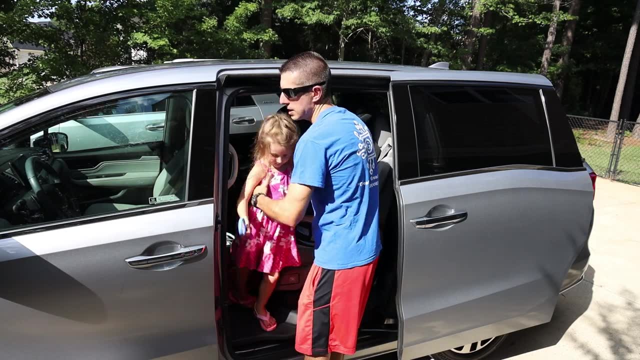 All right. you see that four-year-old that can easily get into the minivan. at three She could get into the minivan. All right, Come here real quick, Come here, All right, let's say. let's say I was just putting her into her car seat, so I pick her up and then I would put her in. 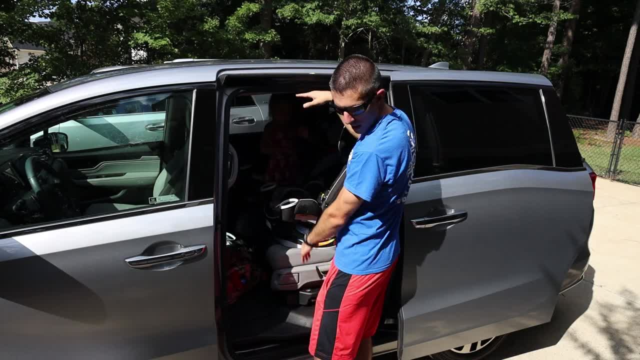 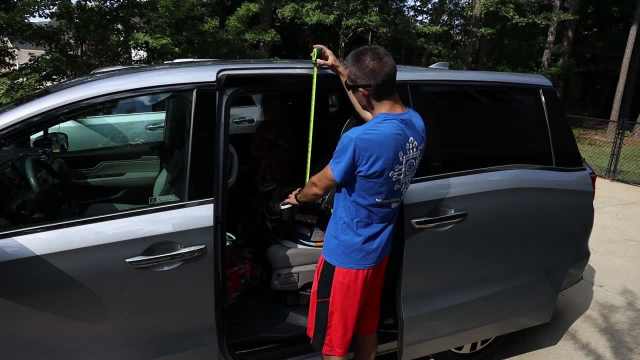 Okay, as you can see, from the car seat side to here There's a good amount, So let's see if I can do that measurement. All right, so from the car seat Armrest to the right here where she would bang her head, is 21 inches. Okay. 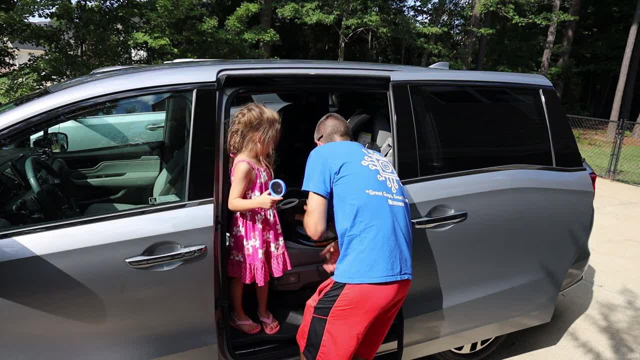 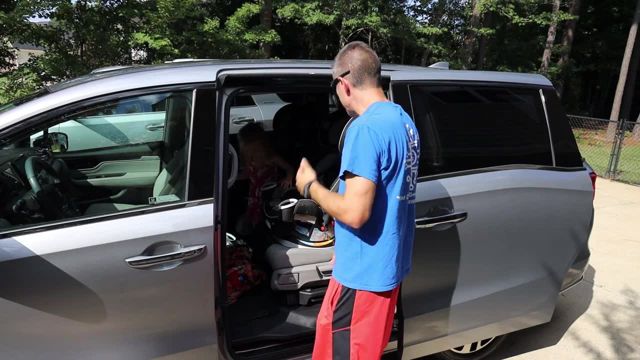 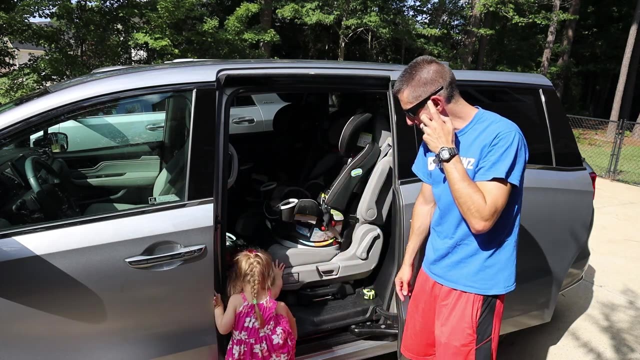 All right, come here. come here. All right, I'm gonna get my second volunteer to show you a little bit here. come on, You'll get you get it. Okay, go ahead, get up in there. All right, two-year-old can step up into this minivan, No problem. 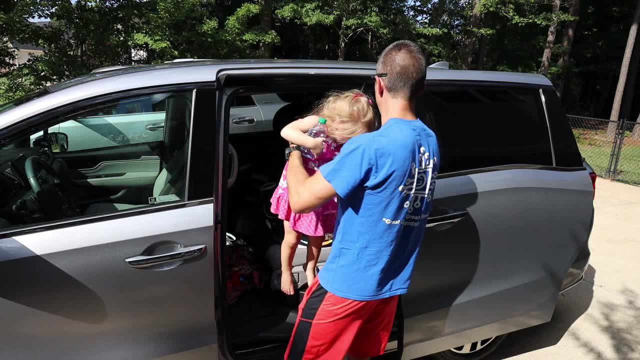 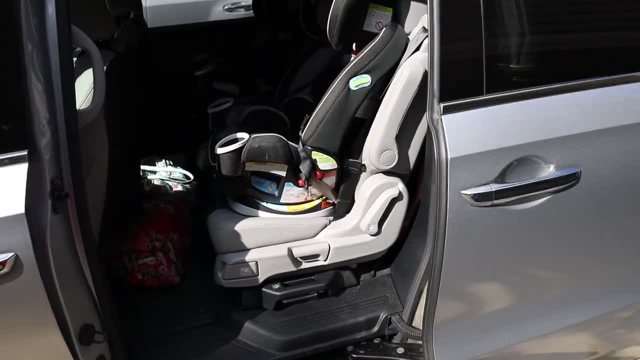 She's obviously got her water bottle here, so if I'm gonna pick her up and put her in, as you can see, There's a ton of room To go over the sidewalk here to get her in the car seats. It's a very nice thing. 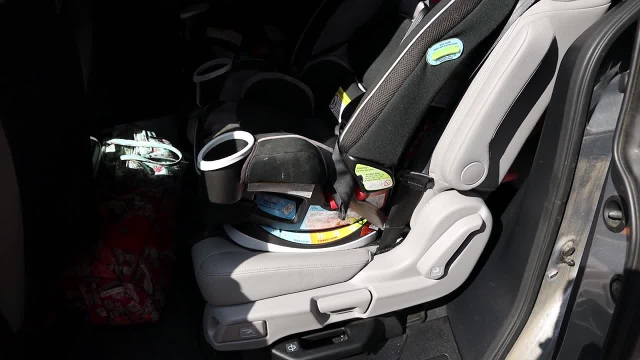 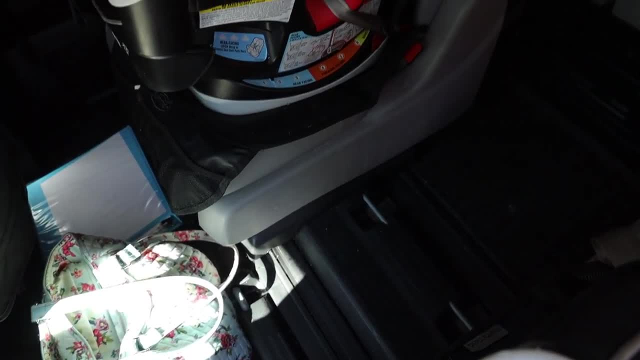 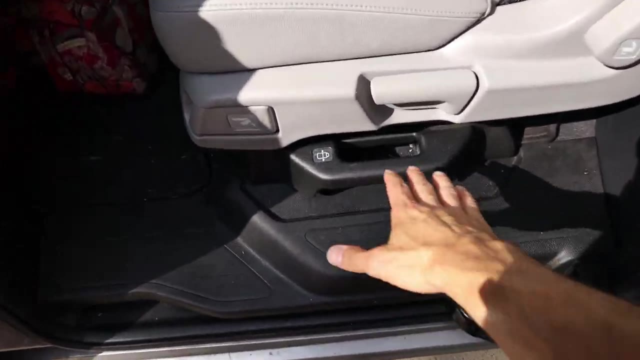 with this particular model odyssey. all the odysseys, the new ones do it. as you can see here in the middle, it is missing that center seat. there's a good reason for that. these are two captain's chairs. I always leave that center seat out for this particular reason. right here you're. 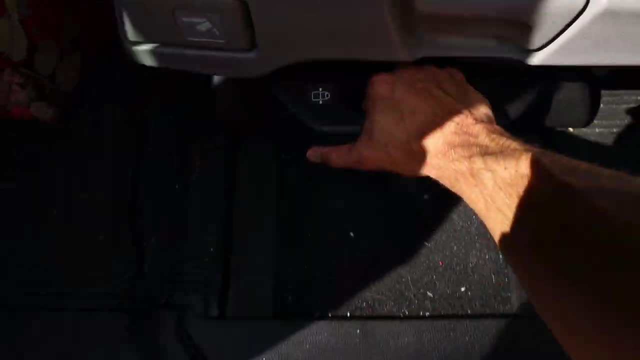 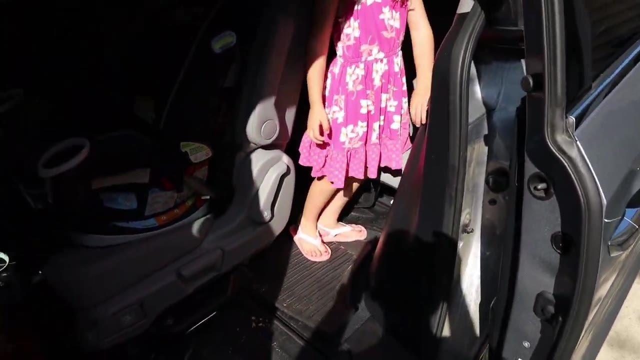 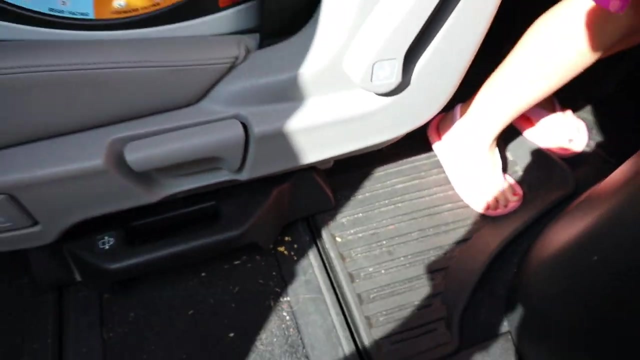 down here. you just there's a grab handle, you squeeze it and slide it. okay, so that way anybody who wants to get in the back can easily just scoot right in the back. with that side seat folded, you can also move them to where the both seats are in the center, like that, and then the other. 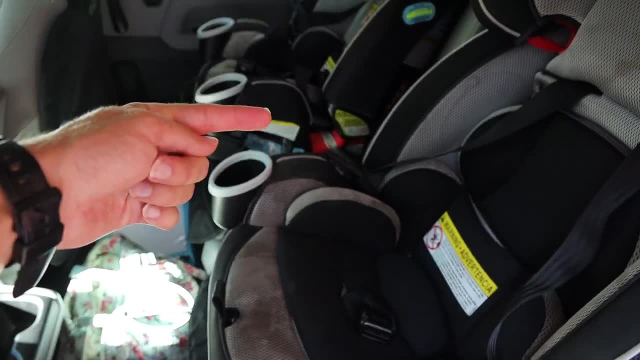 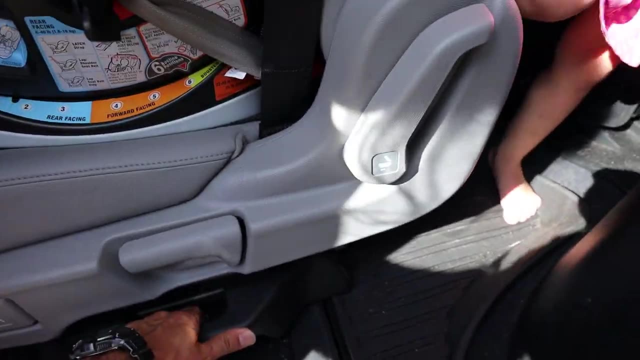 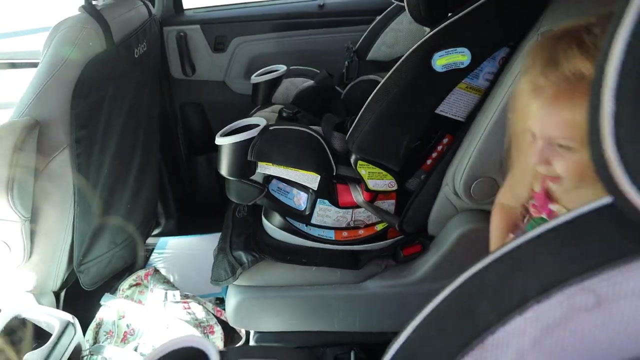 one. you can slide it closer to this one. you can configure these in any way you want, but obviously if you have that center seat in there, you can't slide this. it's back in there now, all right. so that is one great benefit to the mini oh. 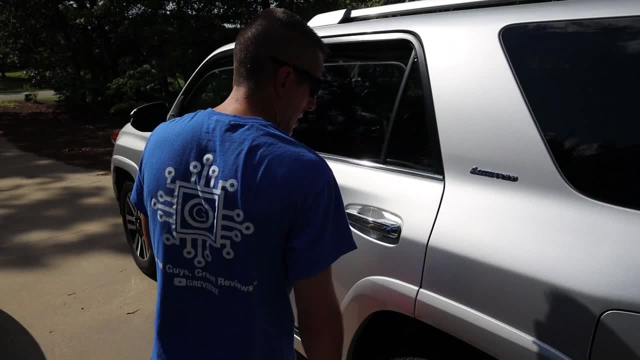 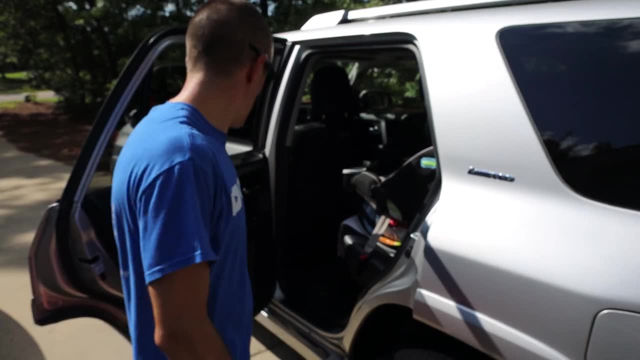 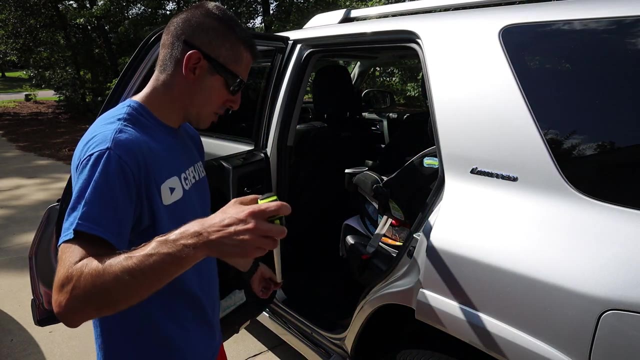 on this forerunner here. the only way to get into this back door is with the handle. all right, no big deal it. it doesn't need to be powered or anything kind of like that. all right, I'm going to get my tape measure and I'm going to measure these dimensions. okay, this is a 15 forerunner. 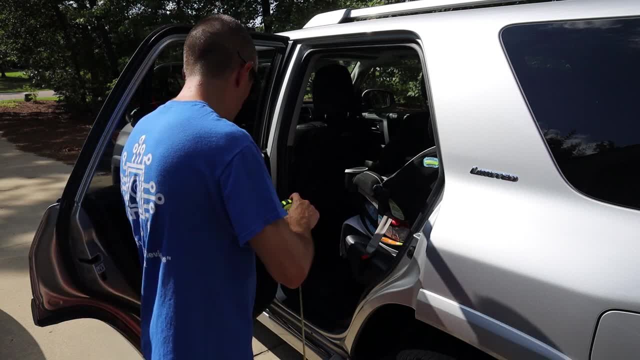 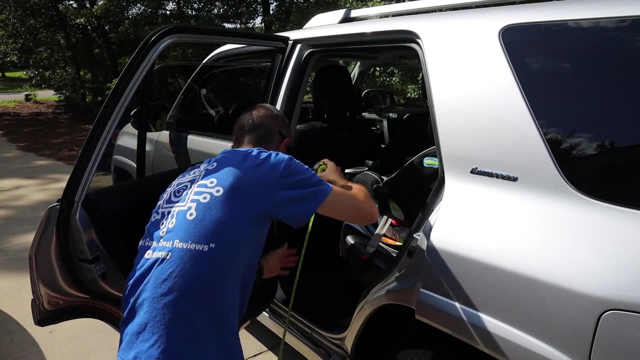 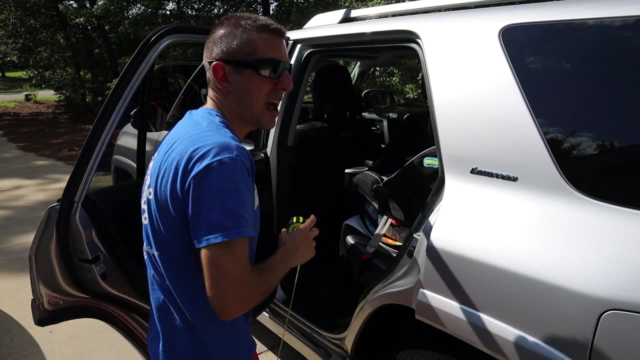 okay, it's got the 20 inch wheels. it's still limited. all right, I'm going to measure from the ground up to the step-in height. all right, step-in height on this one is 21 and a half inches. all right, I believe the other one was. 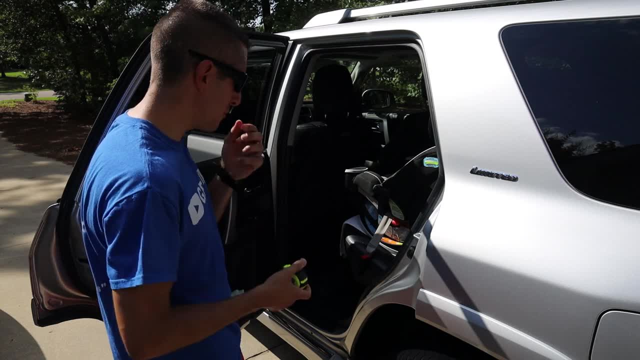 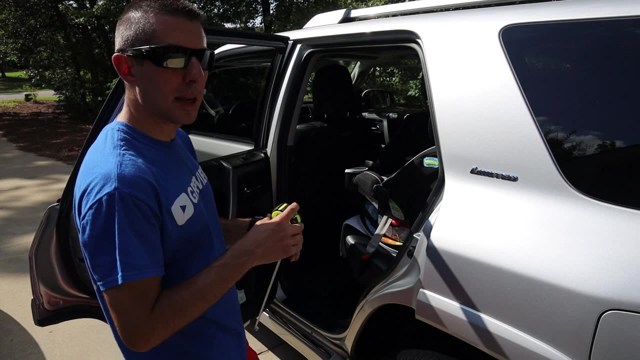 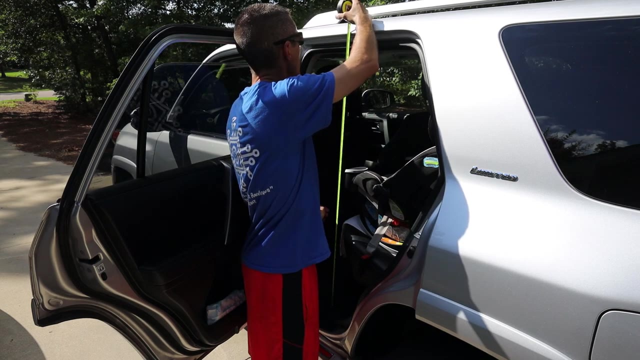 15- I have to look back, correct me if I'm wrong- 15 and this one's 21 and a half. okay, so that's much different, much different. um, my little girl cannot make it in this and my oldest one can barely make it all right: the actual height and the step-in height to where you bang your head on. 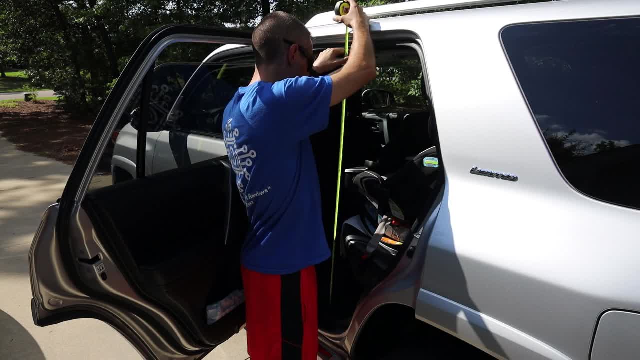 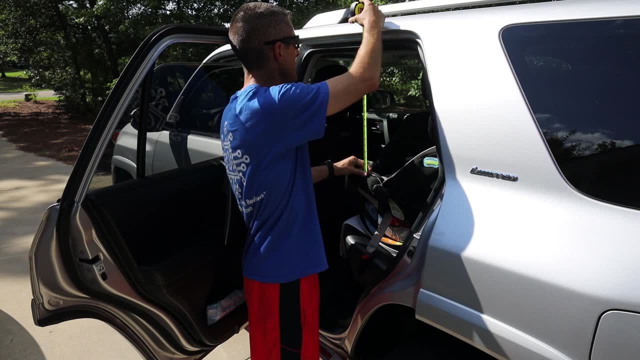 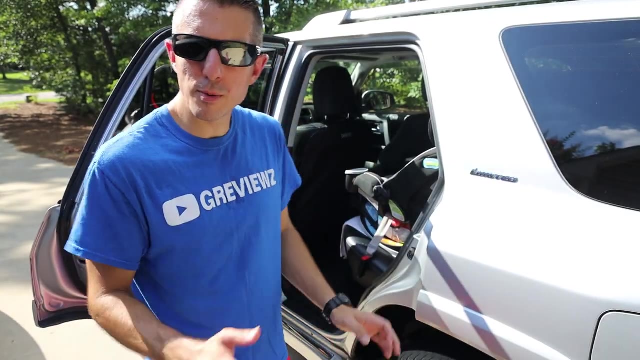 this particular one is going to be 40 two and a half inches, okay, and car seat armrest- to where she would bang her head- is 18 and three quarter inches. all right, i'm gonna go find my volunteers and i will come right back. all right, here's my four-year-olds. all right, get up in there, hop up. 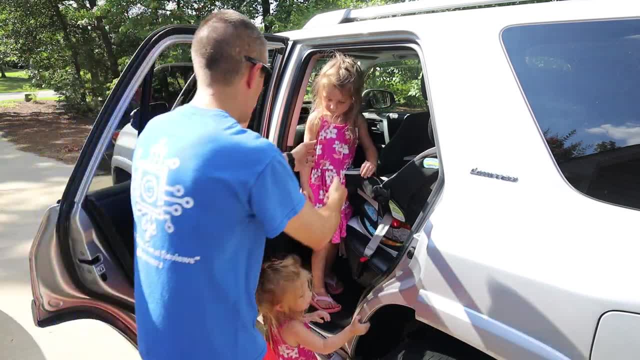 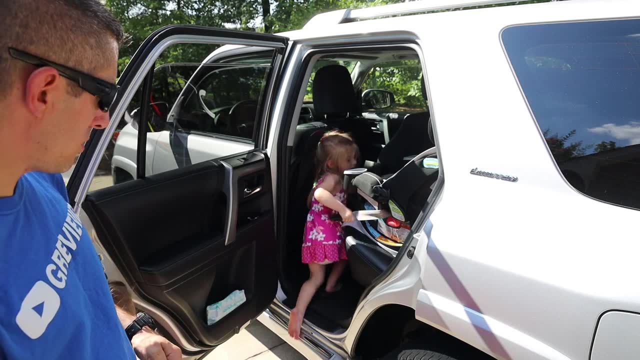 all right, so she can get in. all right, are you hop down? all right, okay, you get up in there. this is my two-year-old. all right, so she both of them could get in. obviously they had to use use the um latch point strap. i don't use that, i just use the actual. 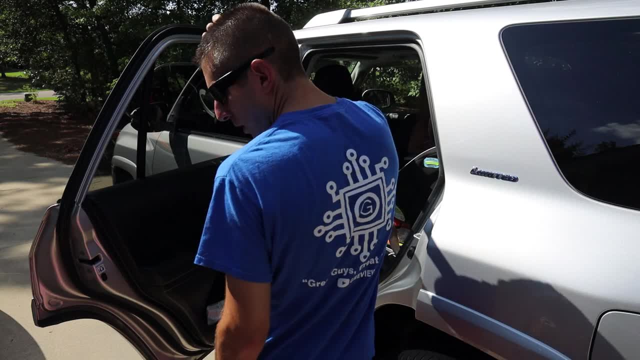 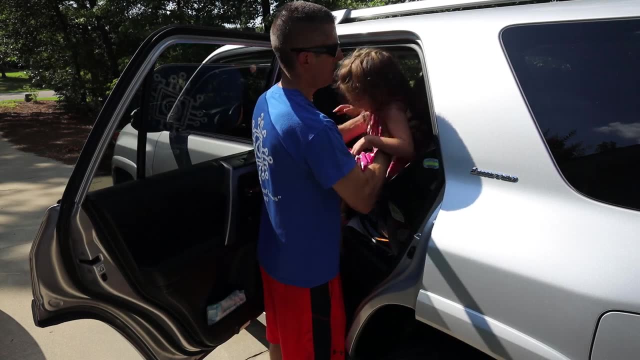 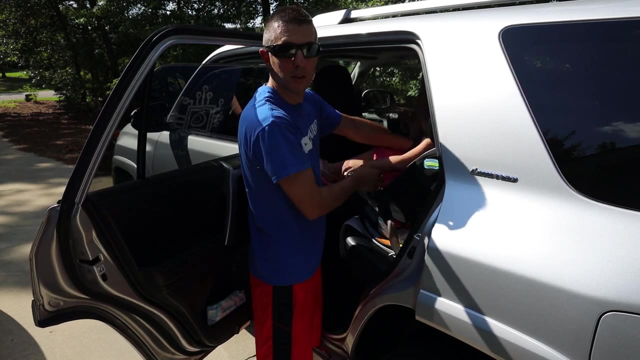 seat belt, which i feel a little more secure with. all right as far as lift up goes, all right, lift her up. all right, see this right here. when i put her in, she's pretty much whacking her head every time i stick her in there. okay, all right, and with my little one, i don't know if she's going to um. 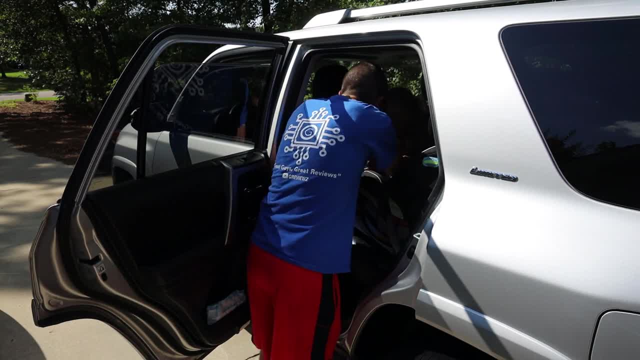 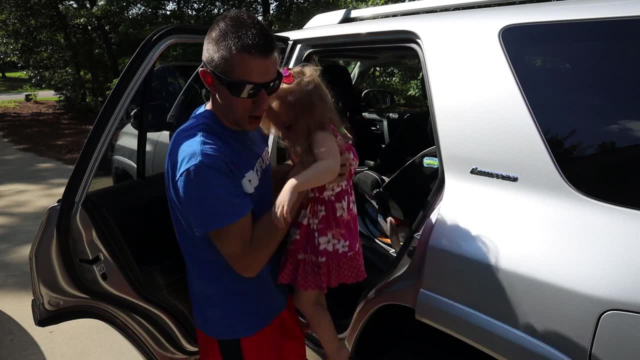 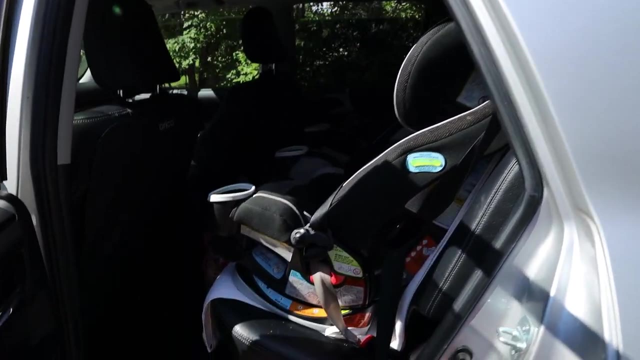 cooperate or not? all right, here's my little one, my little two-year-old. all right, i'll put her in, she's okay. all right, you go. girls did such a good job. as you could tell the, the height from here to here is much smaller on this forerunner than it was on the van. all right, another thing, all right. 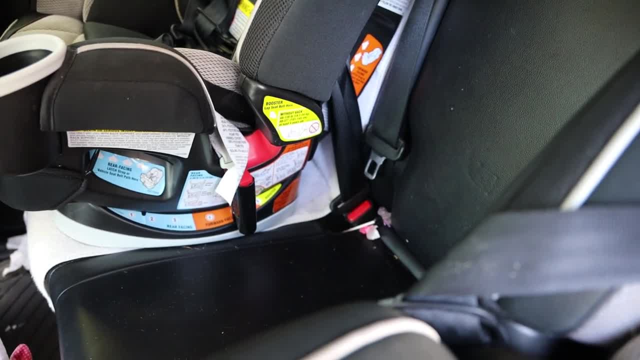 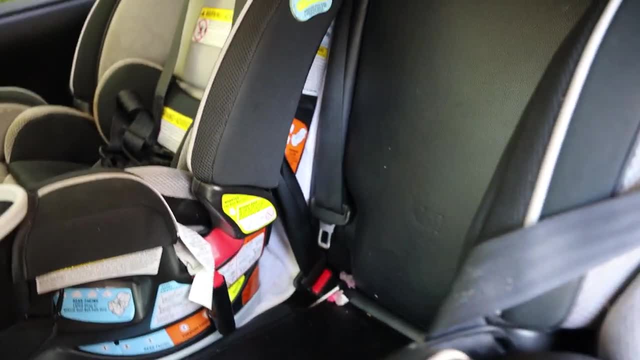 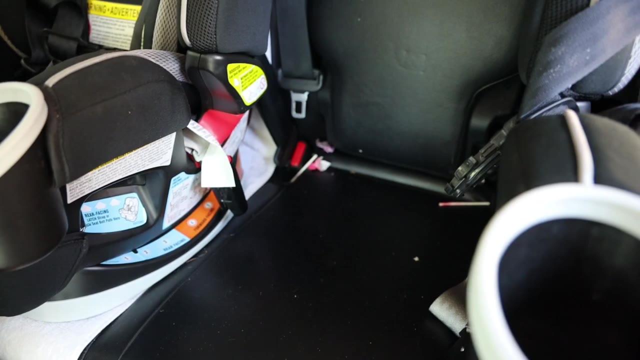 the- both the forerunner and the odyssey- it would be super difficult to put a third car seat in between these two car seats. i mean it could be done. i'm not sure about how safe it is, but you pretty much would have to lean these two seats. 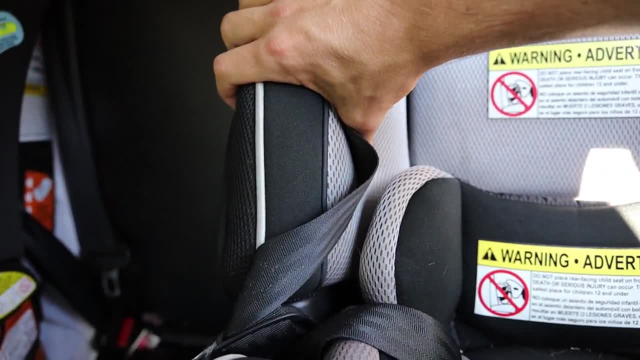 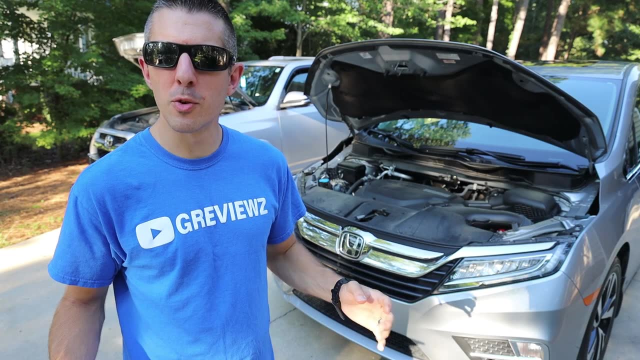 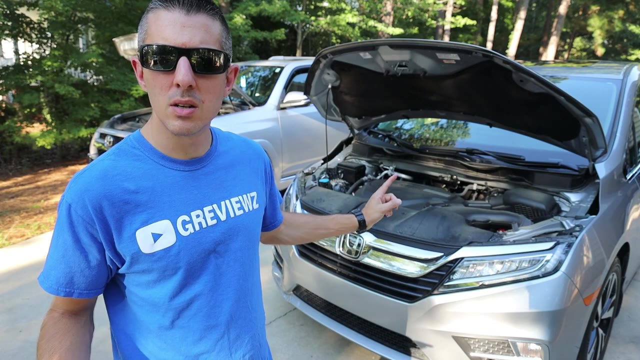 way out like this and i don't know if they'll be pretty secure as those. all right, it's on to towing and miles per gallon- another big factor when choosing a family vehicle for road trips or just a daily drive. all right, let's start with this 2018 honda odyssey. it's got a 3.5 liter v6 engine. 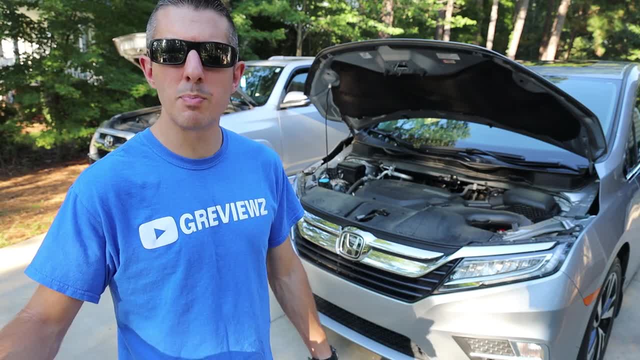 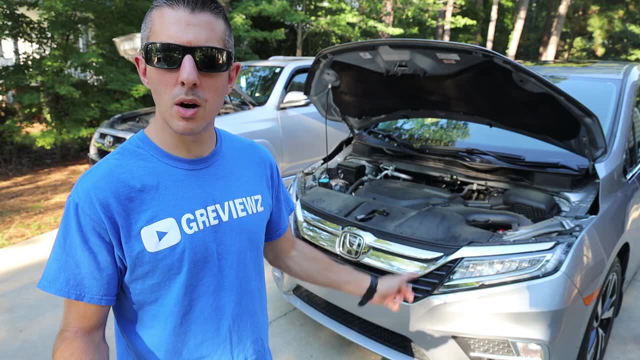 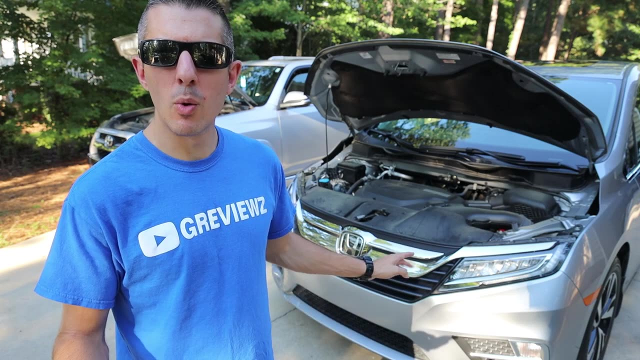 producing 280 horsepower, 260 pound-feet of torque. okay, uh, the towing number on this is 3 500 pounds. it is mated to a 10-speed automatic transmission. okay, it's rated at 19, city 28. on the highway, my wife and i were experiencing about 24 miles per gallon average. okay, now the 4runner over there. 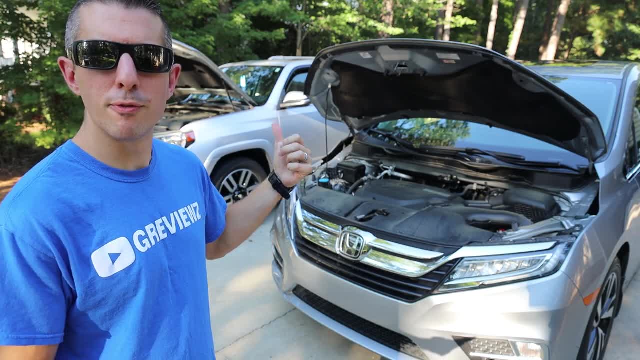 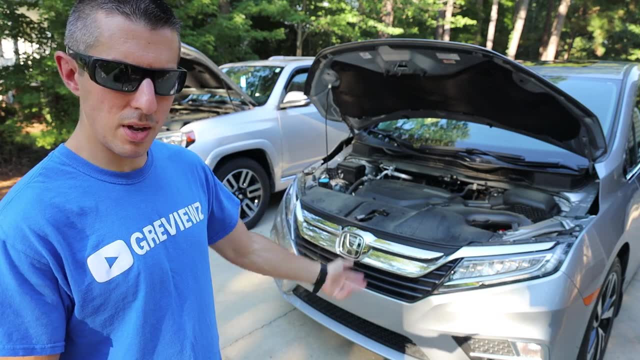 like i said, this is a 2015 toyota 4runner with the standard 4 liter v6 engine. okay, that motor right there puts out 270 horsepower, 278 pound-feet of torque. all right, the towing on that is 5 000. 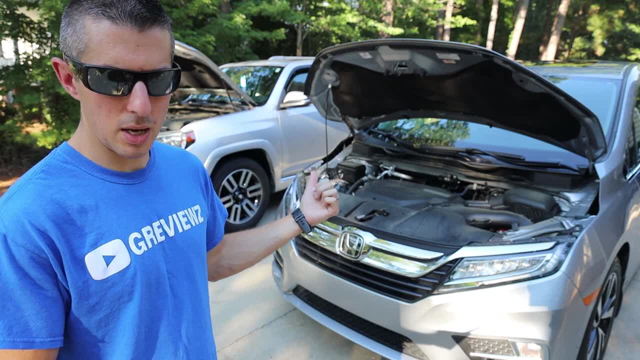 pounds. all right, this is where it's a little bit worse for that vehicle. okay, uh, it's 16 city 19 on the highway. okay. on that vehicle, the engine is about 215 pounds and the torque is about 5 000 pounds, all right, the towing on that is 5 000 pounds, all right, this is where it's a little bit worse for that vehicle. okay, it's 16 city 19 on the highway. okay on that vehicle. 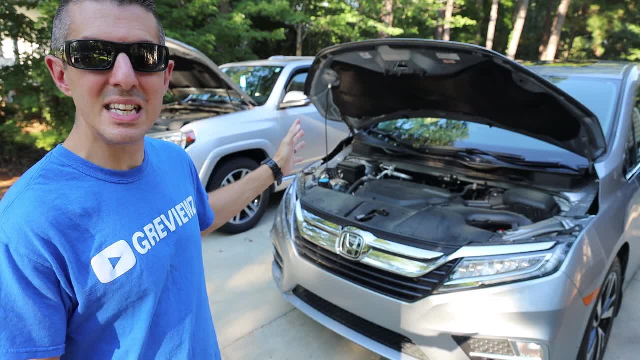 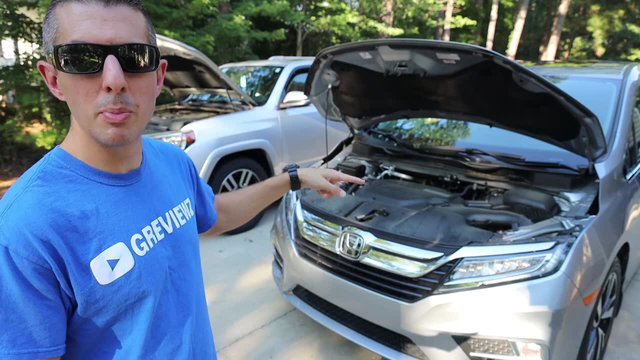 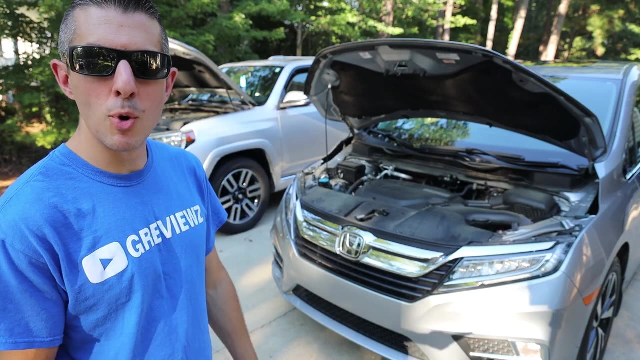 we're experiencing about 19 to 20 average okay. so we think those numbers are a little bit deep, devalued, and we think these are a little bit inflated. I rarely ever see 28 on the highway, even if we just go straight highway driving normally. the most I've ever seen on this is about 26.7 and that's like just 70. 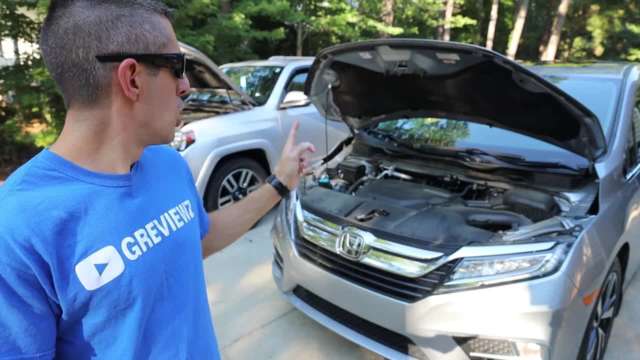 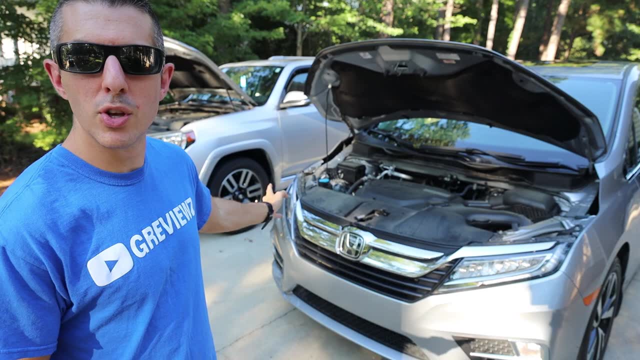 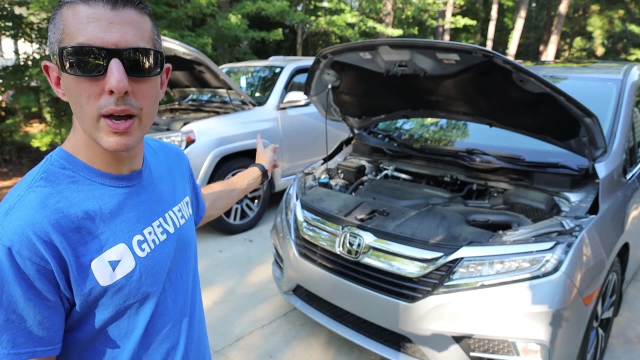 miles an hour. drafting a vehicle where the forerunner is gonna shine its payload. I mean I actually do tow a little bit with that. we have a little utility trailer. we tow like lawnmowers etc on that. there's hardly any squat when you tow light with that. if I fill the back of this up, I mean it's squatting. 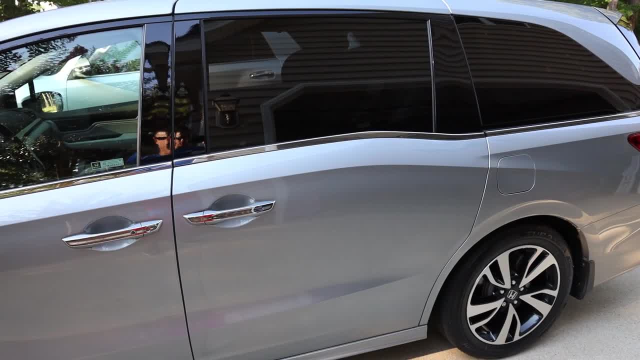 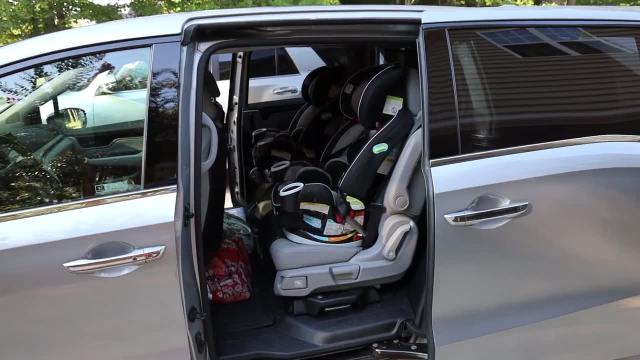 pretty good in the back, so that's something to consider. now I'm gonna go over party tricks. all right, the party trick with this Honda Odyssey is going to be the automatic doors. both the middle door is open. I'm gonna go over the automatic doors. both the middle door is open. I'm gonna 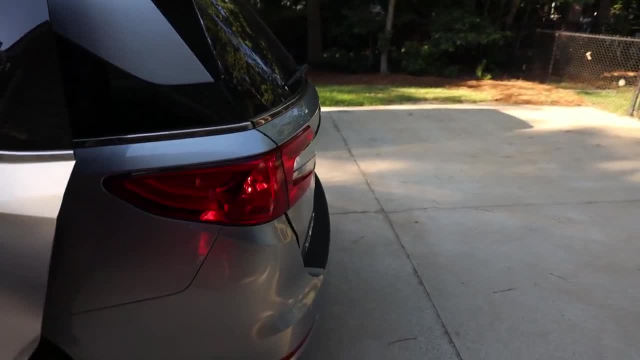 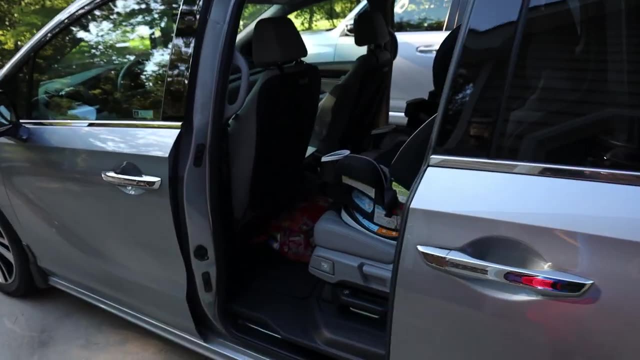 go over the automatic doors both. the middle door is open, I'm gonna go over, and the rear hatch opens all power. I call those party tricks, because that's something a lot of other vehicles don't have. most other minivans have it all right. and then this sliding, the sliding seats- I like that. that's a pretty good. 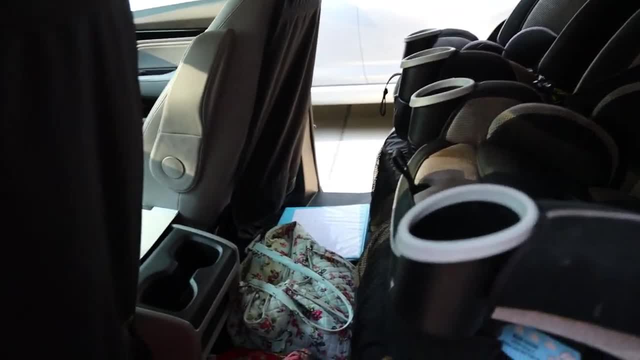 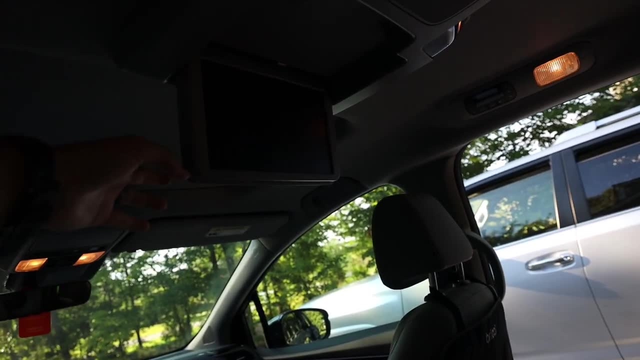 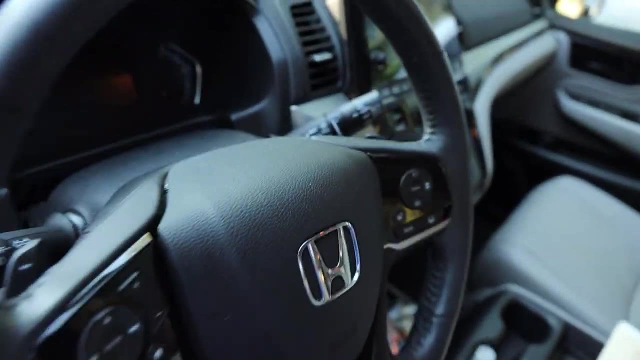 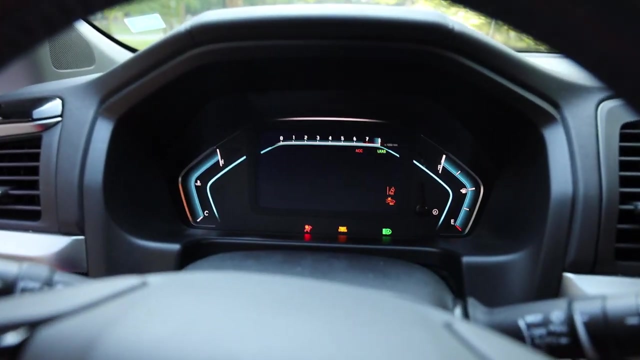 feature. it's not quite stone go like on the Pacifica, the Chrysler Pacifica, but um, it's still still pretty good. all right, it's got the drop-down DVD, all right. another party trick that you have on this Honda is going to be what's called cabin watch. I'm gonna start this up: push button start, obviously the whole. 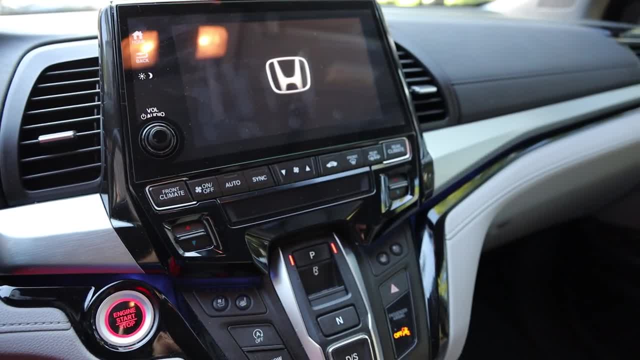 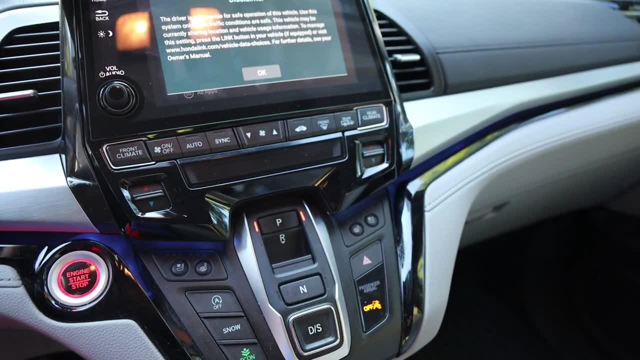 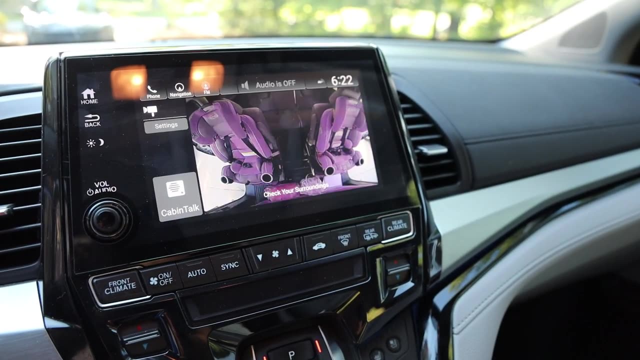 center part there is a screen. all right, obviously the transmission is all push button. okay, let that start up. we're gonna go to home, all right, home. now we got what's called cabin watch, all right, you see that, right there, those are act. that's actually a fisheye lens of. 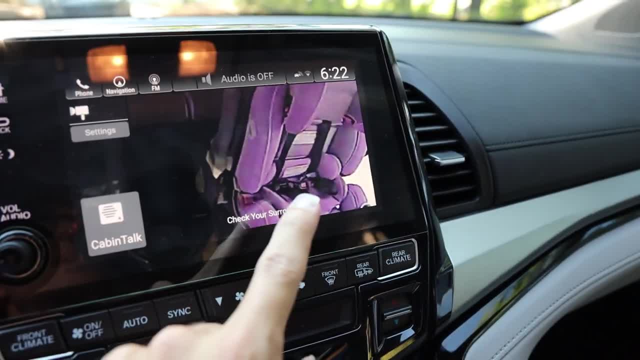 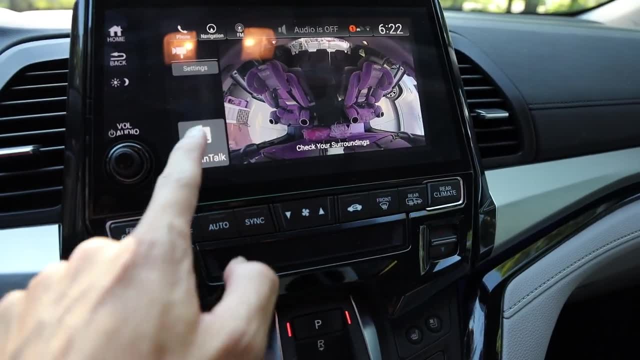 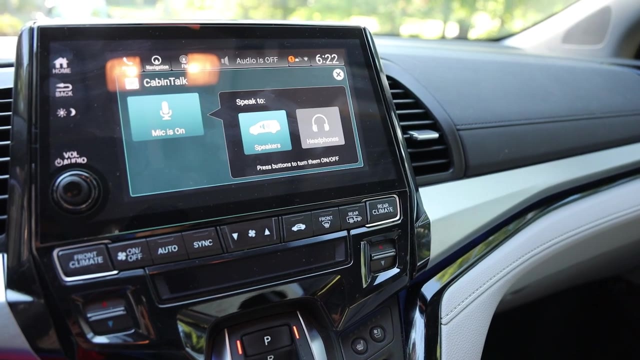 the two kids seats? okay, so I can physically zoom in on one or the other to see who's hitting who, which is great. okay, and now cabin talk. all right, you two cut it out. I don't know if you can hear the echo in the background, but so. 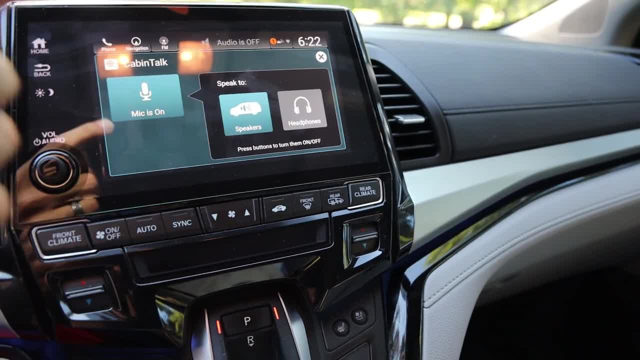 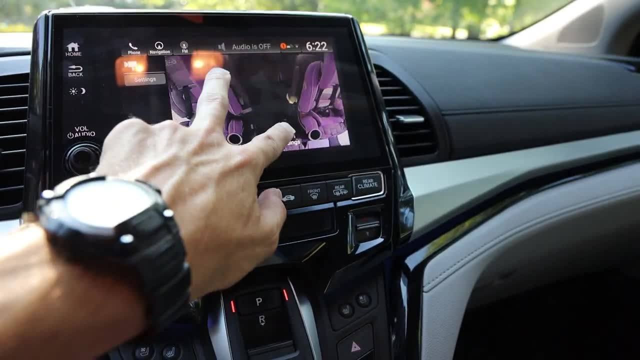 if this kids way in the back of the yelling screaming this actually goes through the vehicle speakers in the back and it's kind of loud back there. to be honest with you, that's. that's an awesome. this is an awesome feature. I mean I can see all the 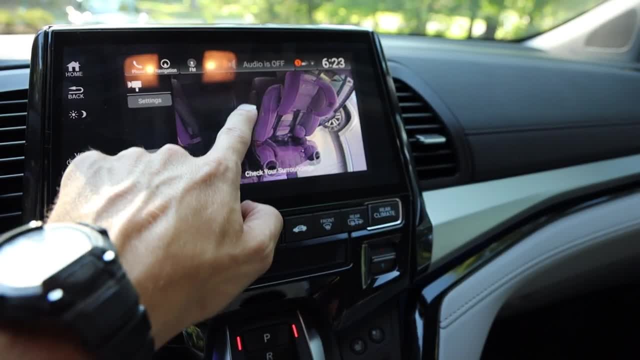 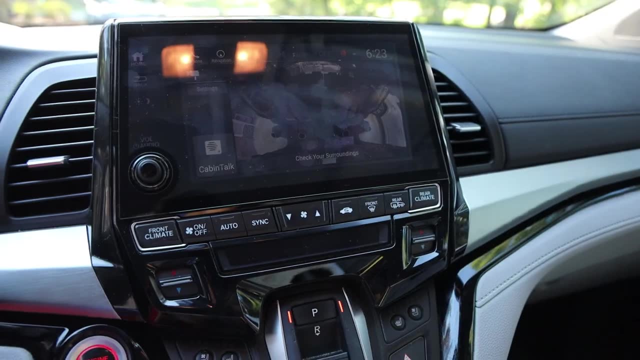 way in the back if there's some hanky-panky going on with some older kids or whatever have you? but all that right. there is a great feature that I really like. that's another party trick. this forerunner has a little bit less in the way of party tricks than the odyssey. 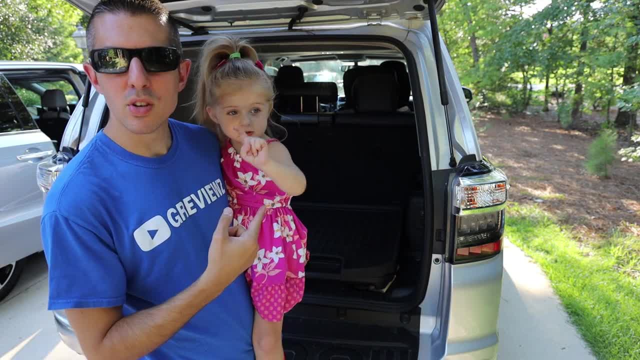 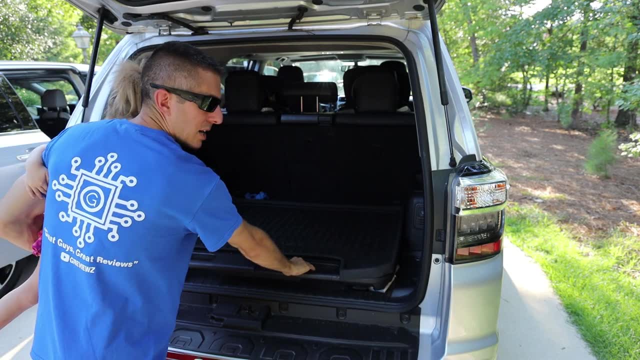 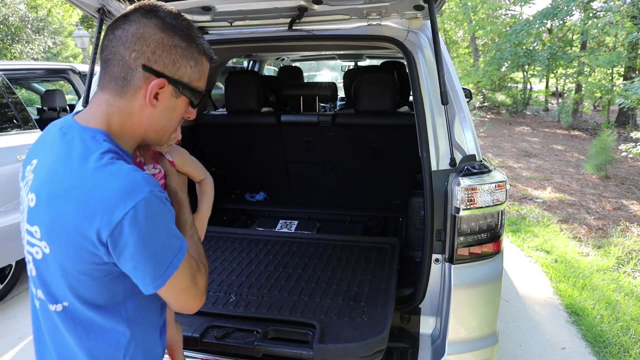 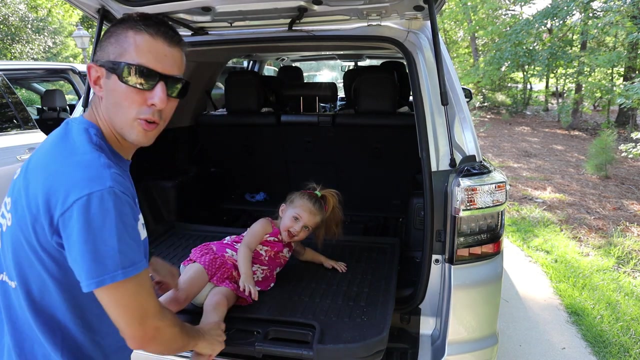 does. however, one big selling point while we got this is for the built-in change table. let me show you example. baby, nice sliding tray comes out approximately two feet past the actual bumper area. now check this out. okay, long story short, you don't want to do it, but this is a nice waist-high changing table that we've. 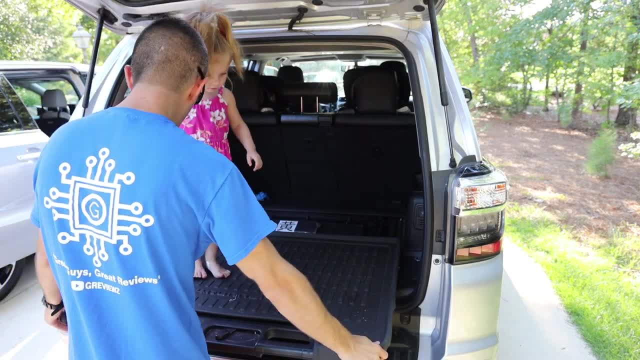 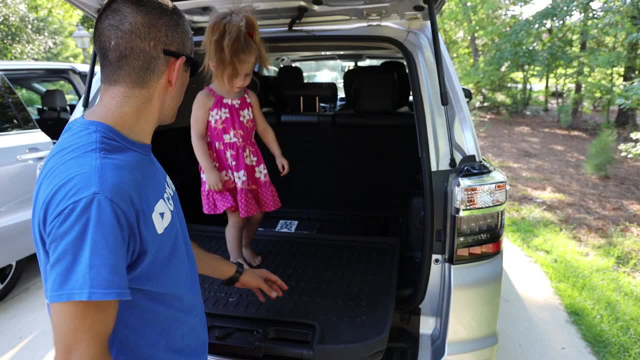 used on both of our girls. it's a great place. um, like I said, it's got this nice, uh, pretty much like a weather tech mat, so it don't matter if it gets whatever on it. it's a great for that. all right, you're done. you can go back in the house. 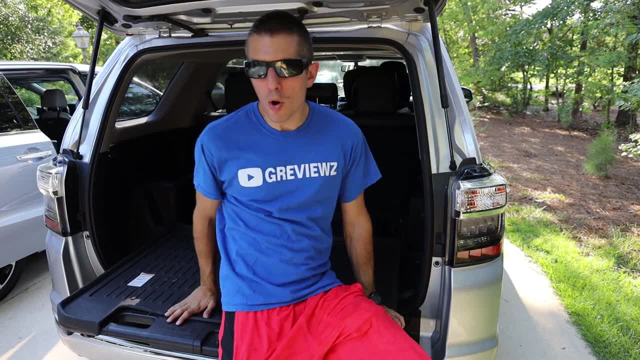 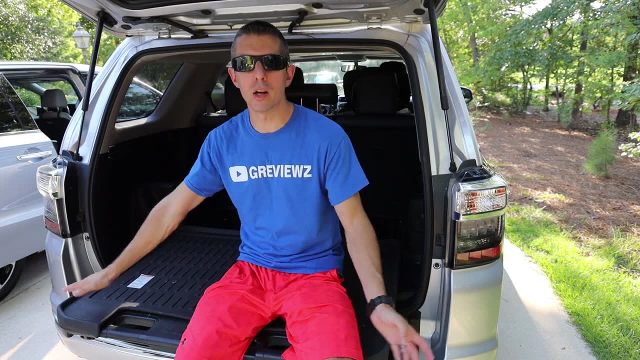 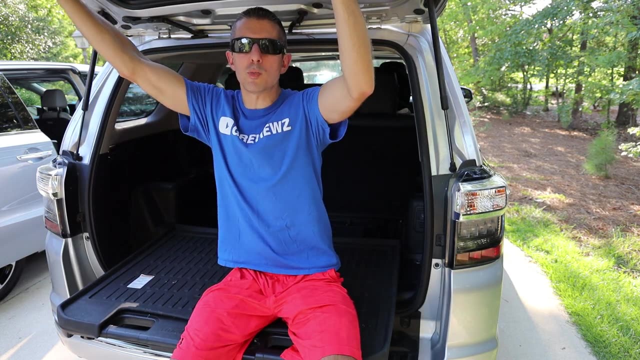 all right, thank you. like I was saying earlier, another party trick to this is the fact that this thing holds 440 pounds slid out. so me and the wife and the girls all have sat on this at some point, like if we're at the beach or whatever. have you? and right up here in the door are actually two nice speakers. 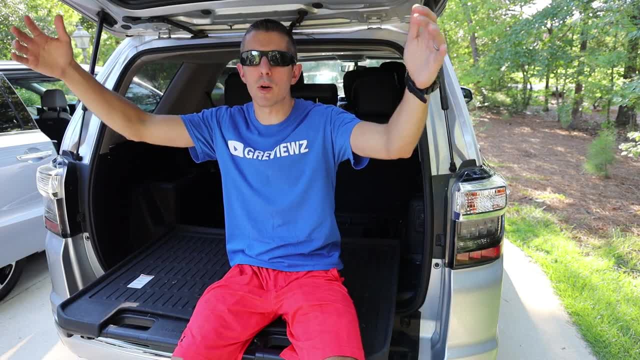 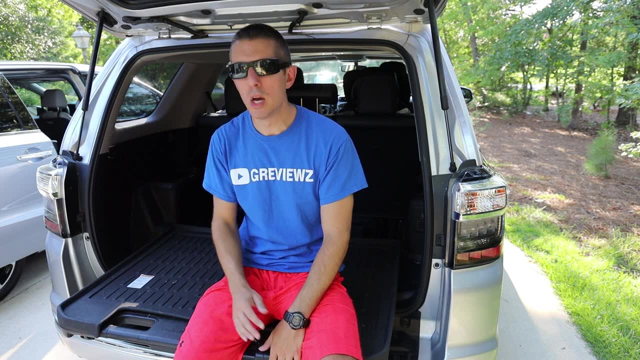 so if you're sitting out here, you know obviously I'm in the shade. right now it's super hot out here, but with the shade it's nice and with the speakers right above you it's a nice little party area back here. you could actually. we've actually cooked on this. 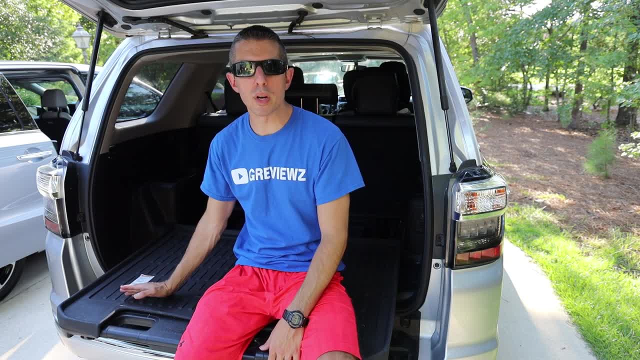 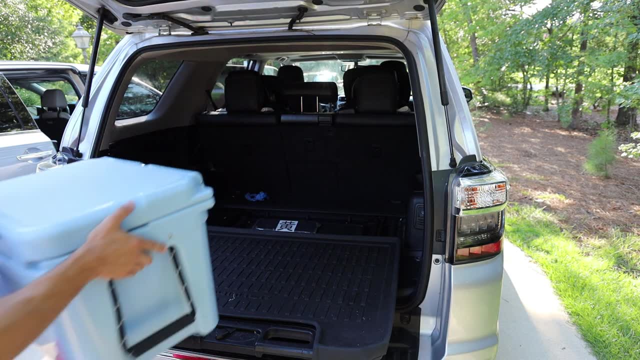 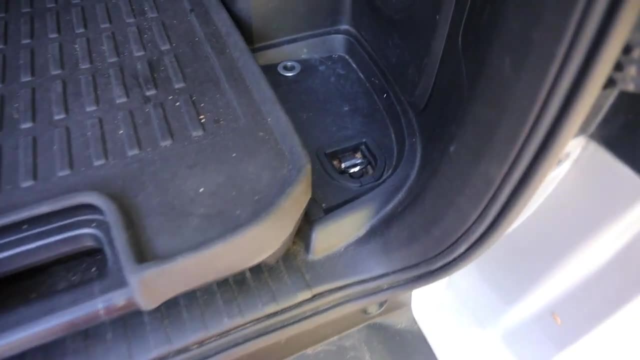 for camping. we put a little Coleman stove right here. um, you could put drinks, whatever have you. it's just an easy thing to where you can put heavier objects on this, for example, like that, and then you can slide it back so you don't have to lean so far into the vehicle. as far as storage goes, I like the fact that the 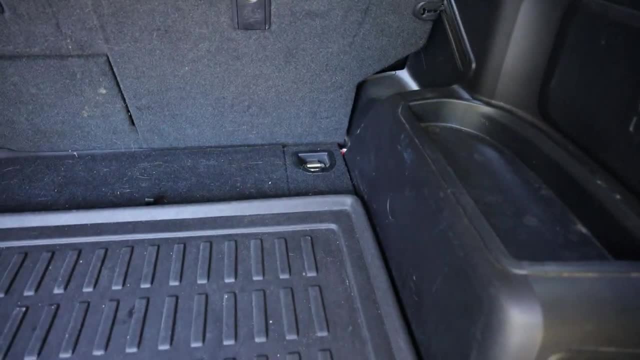 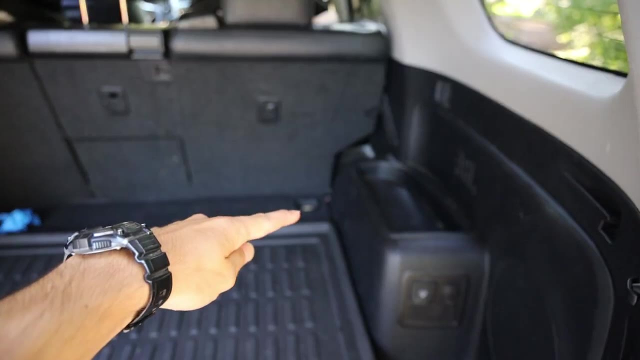 forerunner has four tie down cleats in the corners in this vehicle. Okay, what that allows you to do is to stack things higher up, And I used to use a strap and strap over top of the object so they don't move around. 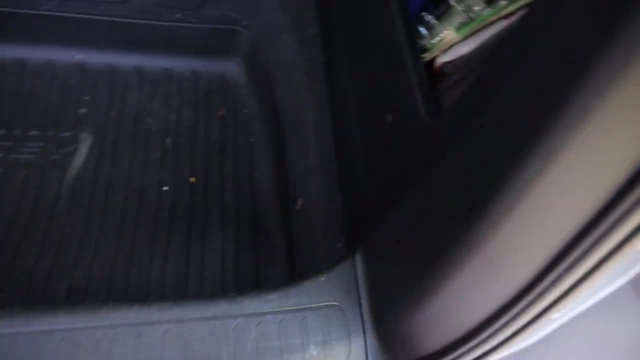 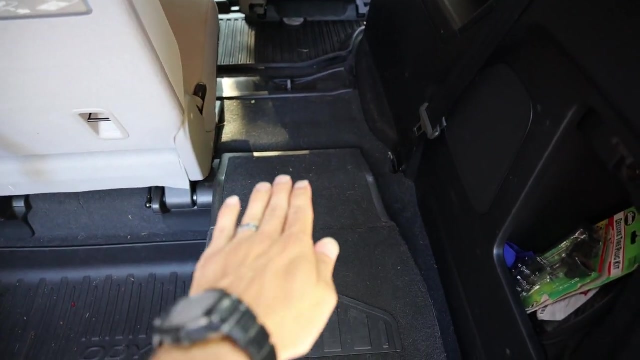 All right, in the Odyssey there isn't a single tie down point to be had. okay, All right. so even when you have stuff in here, this actually has a slope going downward into the vehicle. So if I ever put something back here, 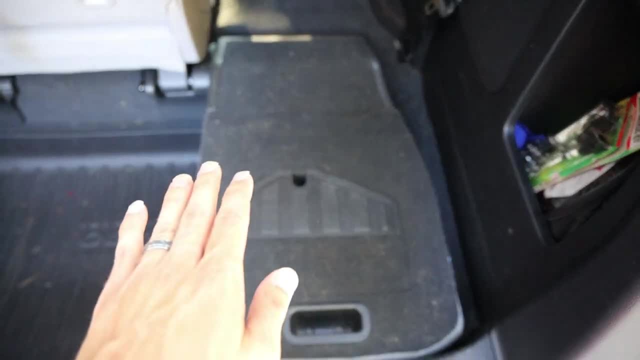 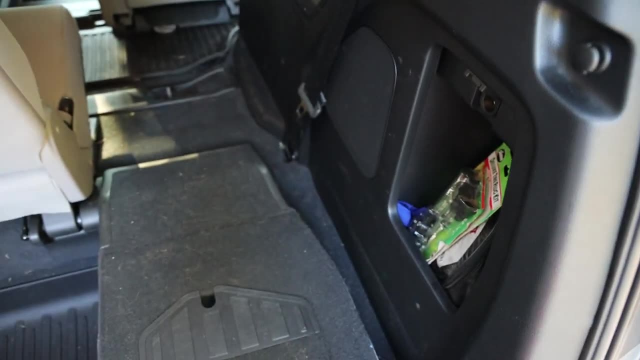 for example, a cooler other than the Yeti with the rubber feet, and I would hit the brakes. everything slides forward. Like I said, there's no tie down cleats or tie down points anywhere in this van, which is a negative in my opinion. 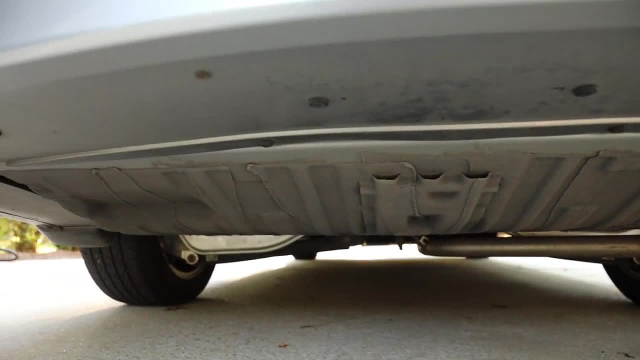 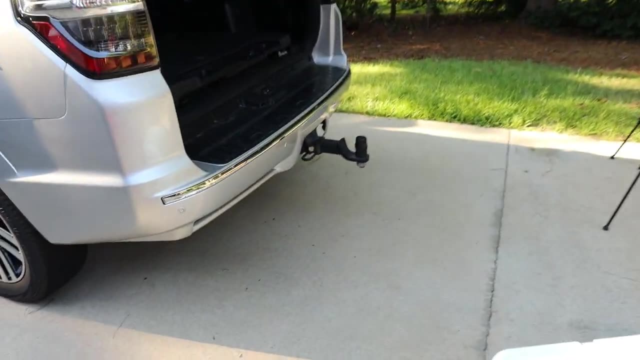 As far as the hitch goes, I mean, I've seen people with hitches, but it's kind of a pain. all right, On the 4Runner it's already built in with the hitch receiver. I know this is a little rusty looking. 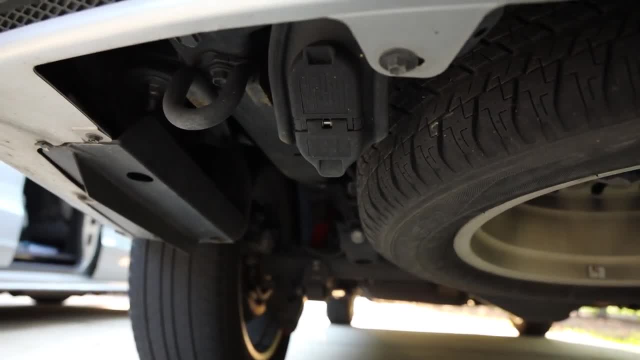 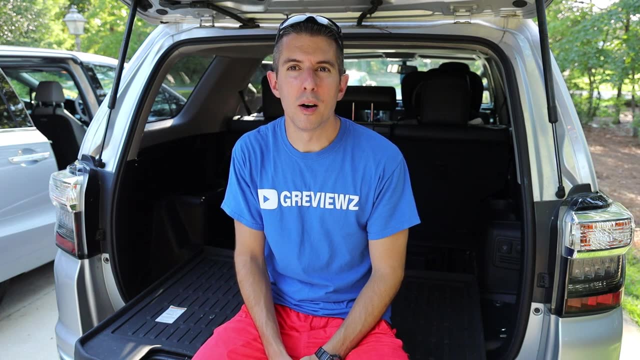 And it also has the wiring pin down over here. Hopefully you can see it. All right, I'm gonna drop some conclusions and you guys can take it for what you want. Both of these vehicles are great family vehicles, Don't get me wrong. 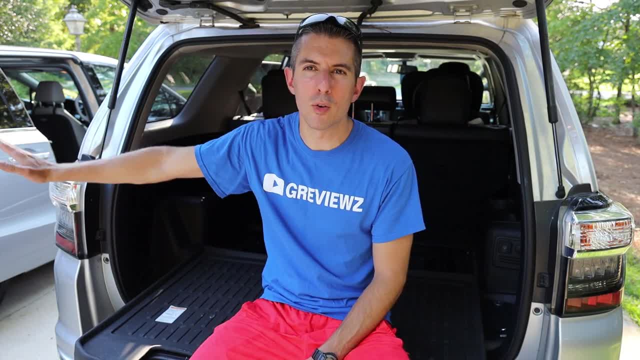 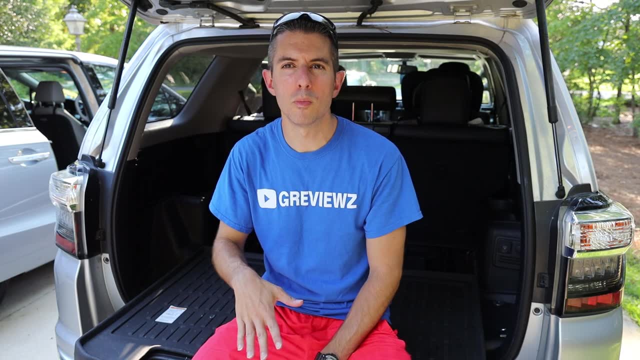 Like I said, we own both. We own this 4Runner, We own that van over there. Obviously, this is mine and that's my wife's. We started out with this 4Runner before we had kids, thinking it was gonna be big enough. 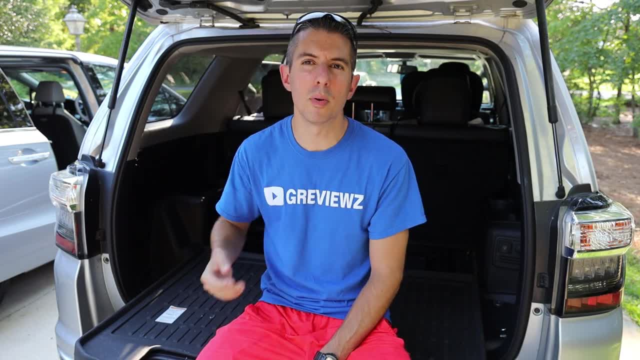 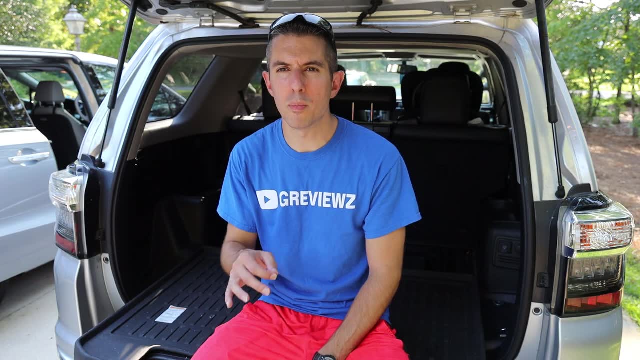 We have two kids now, So obviously the inside's pretty much taken up This back. I have another larger cooler. It's like a 70 quart cooler That, with my full size golden retriever back here, takes up quite a bit of room. 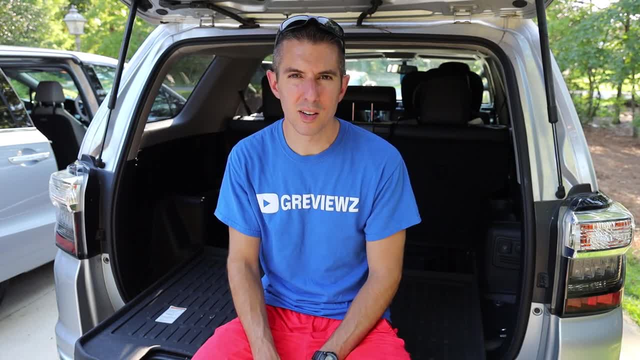 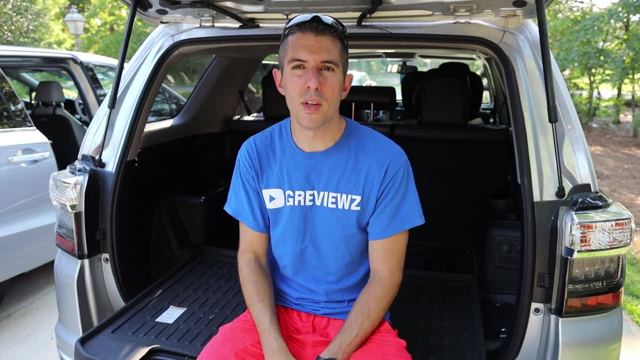 So this vehicle got a little on the small side quickly. That's why we ended up with that Odyssey over there, because it's got physically more storage than this 4Runner does. Now if you're looking to get one or the other, you have to pretty much think of. 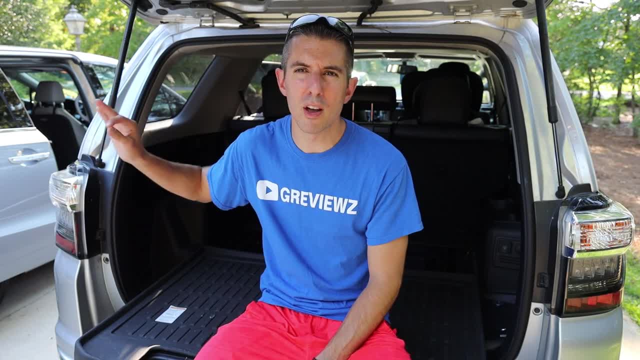 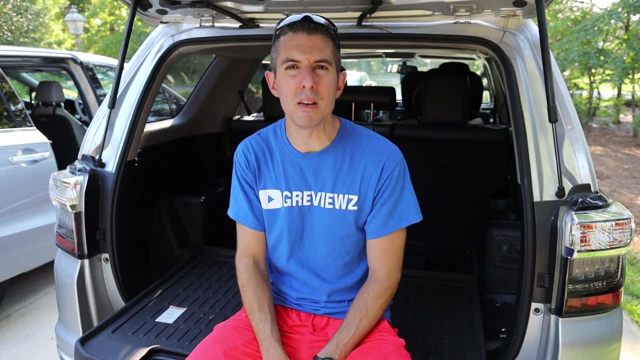 if you want ultimate child family vehicle, that's going to be the Odyssey. If you want a great family vehicle that can take you off the beaten path. so, if you wanted to go on the beach, drive on the beach, go off road, anything like that. 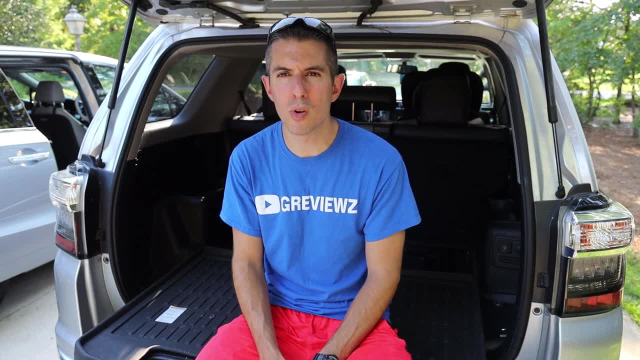 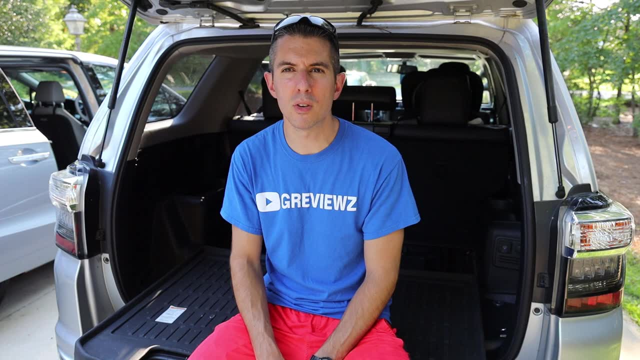 the 4Runner is the vehicle for you. If you wanna tow a small camper or anything like that, I would definitely go with the 4Runner. Now, if it's just a point A to point B- soccer mom type vehicle, the Odyssey is gonna be for you. 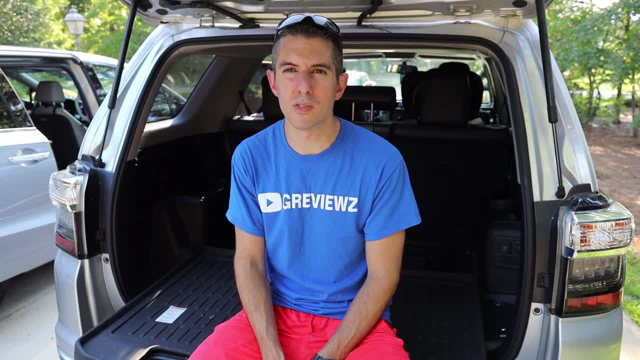 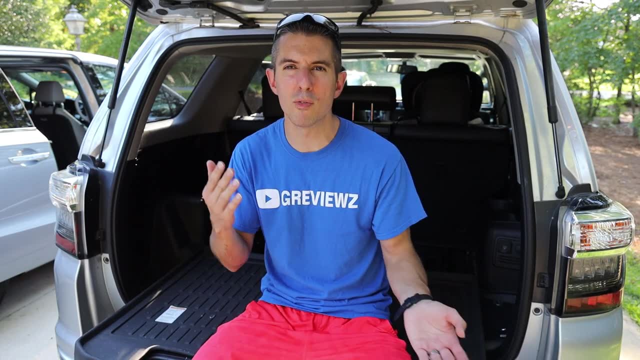 So, guys, that's my conclusion. It all depends on what you value in a vehicle. Please leave some comments in the description below and tell me: what do you guys rather have? Would you rather have a SUV, or would you rather have a minivan? 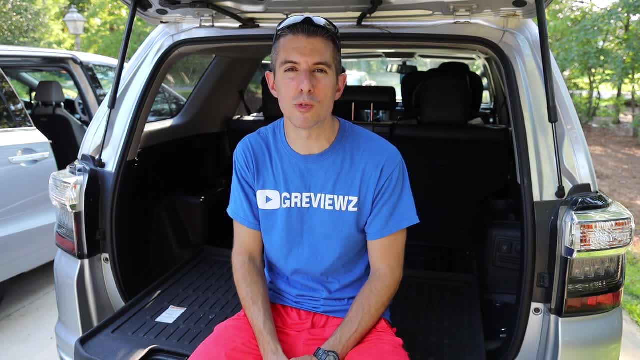 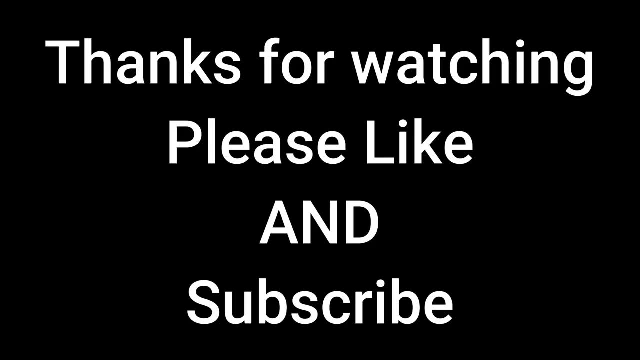 Obviously, I can't make that decision for you, but hopefully I presented you with some good arguments. All right, you guys have a great summer. I'll see you in the next video. Bye.